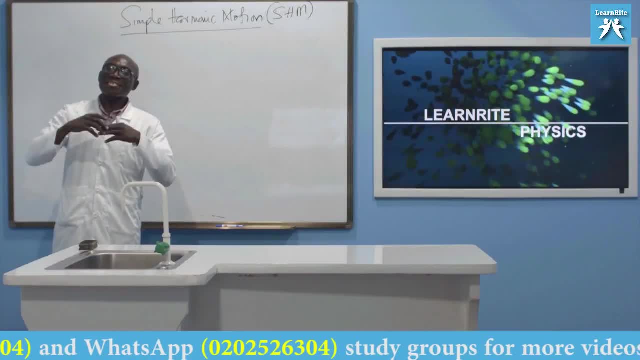 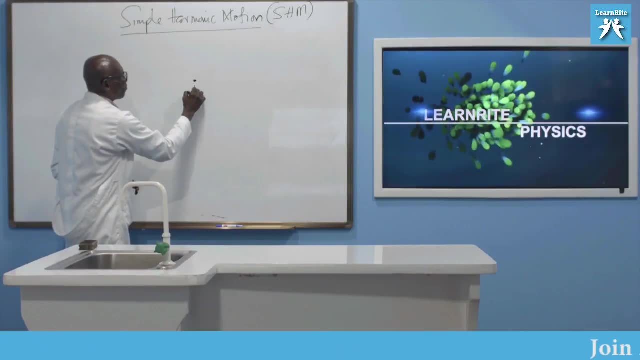 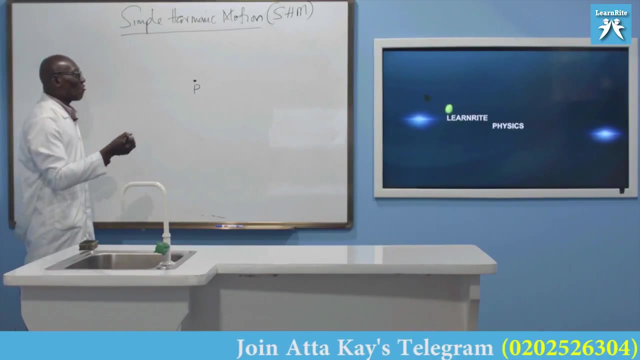 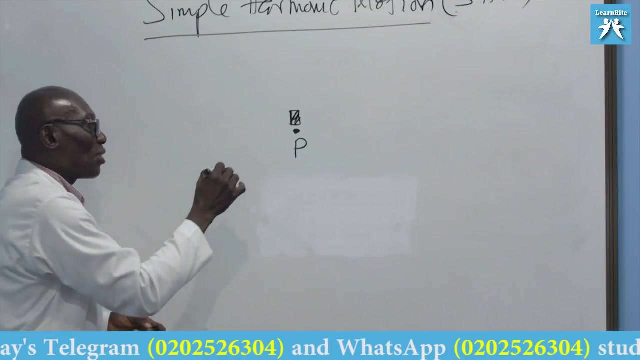 SHM, SHM. So what is simple harmonic motion? Let me take a point P and call that point a fixed point, And I have a body At this point. we call it a fixed point. Now the body moves away from this fixed point. 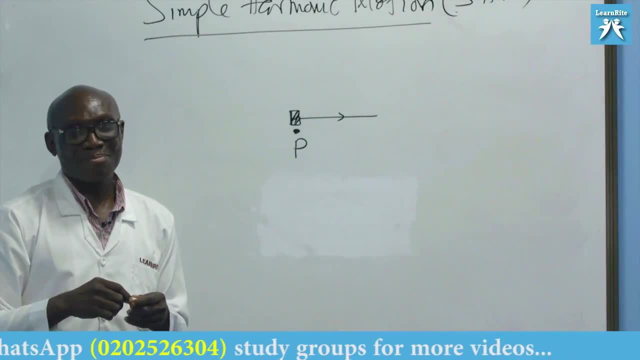 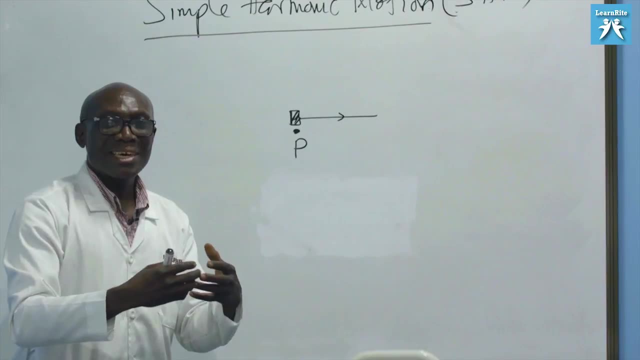 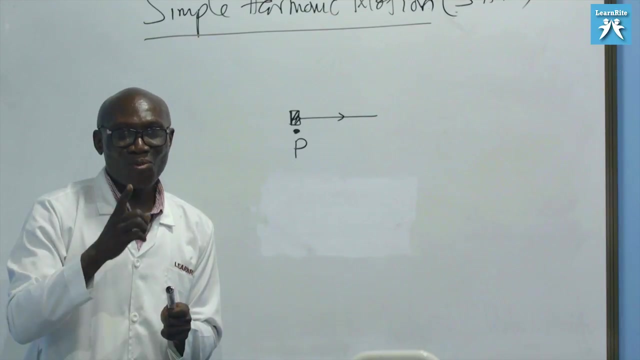 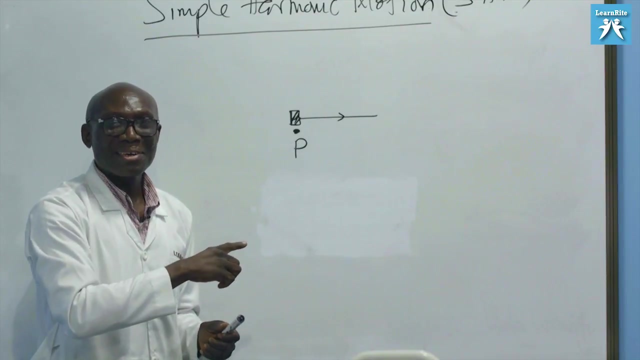 And that body does so with an acceleration. Why? Because the body was inactive, The body was initially at rest and the body moved and gained a velocity. There has been a change in velocity, so the body possesses acceleration. Watch this: The body is going away from the fixed point. 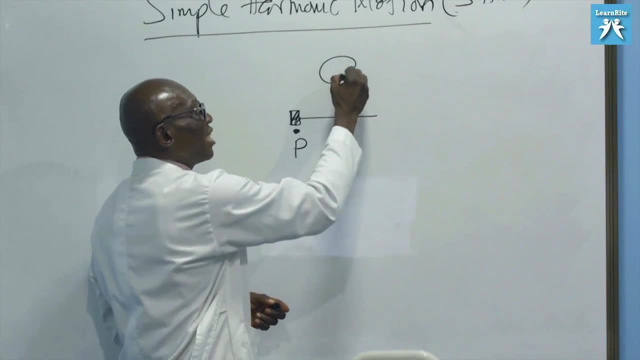 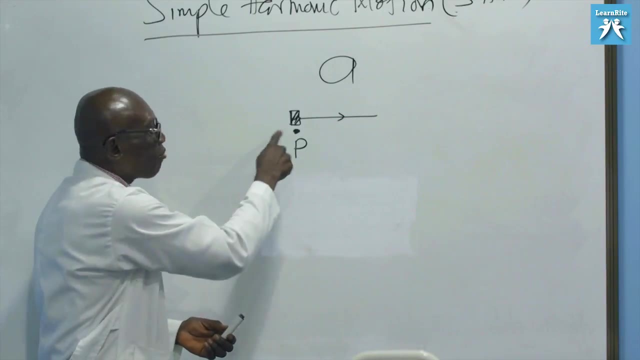 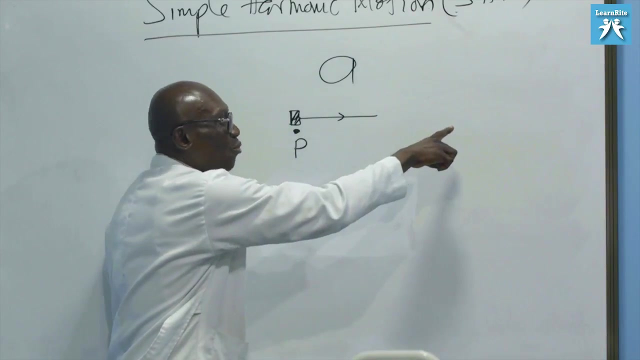 But its acceleration, its acceleration- I'm using A for that- its acceleration is rather directed, directed towards this fixed point. So strange: The body is moving away, This direction of motion, and yet its acceleration is drawing or directed towards this fixed. 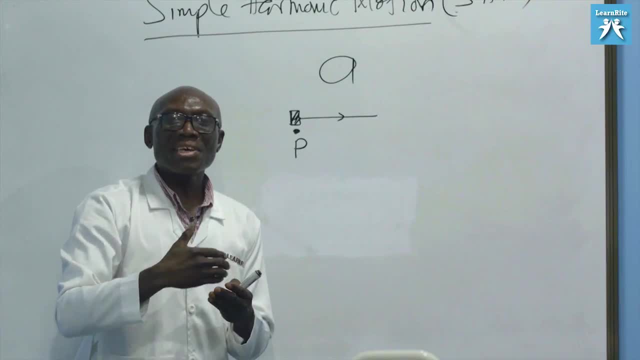 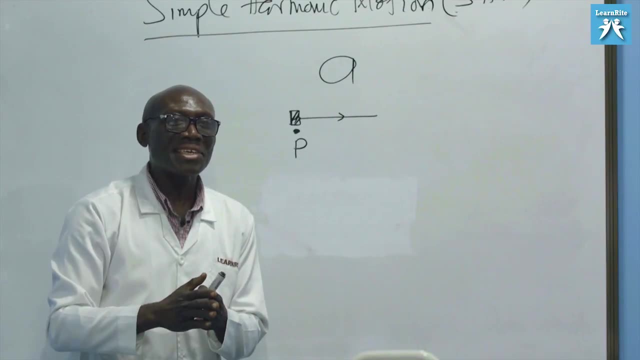 point, And let me say this: Force gives rise to acceleration, and so force and acceleration are in the same direction, And so what it means is that the force on this body is also directed in the same direction, and you look at the affects on the environment, you don't know what that mean. 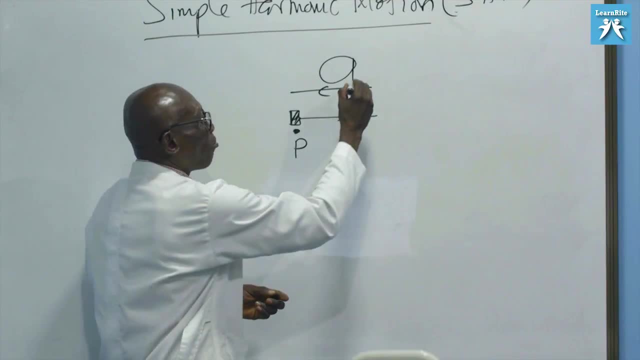 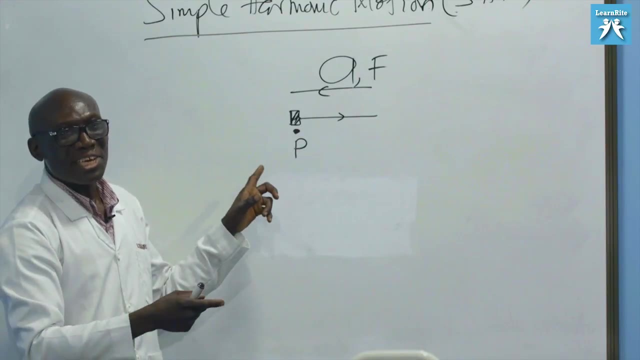 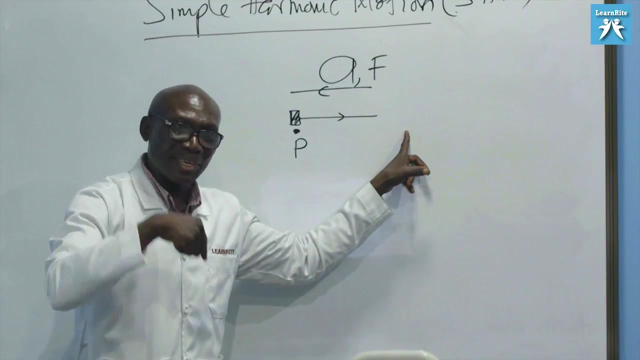 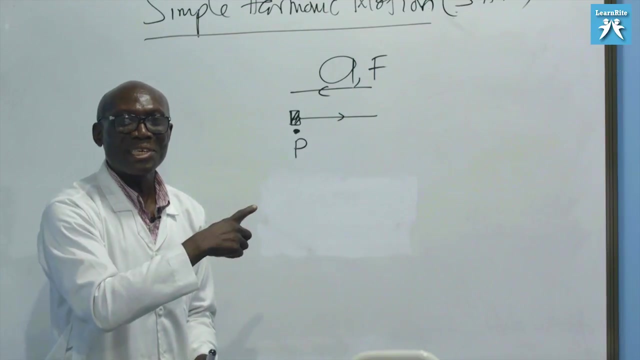 same direction as the acceleration. So we have both the acceleration and the force directed toward this fixed point And, I repeat, the body is moving away from this fixed point. This is the direction of motion, and yet its acceleration is directed toward this fixed point. It means that the force on this body will also be directed toward the fixed point. 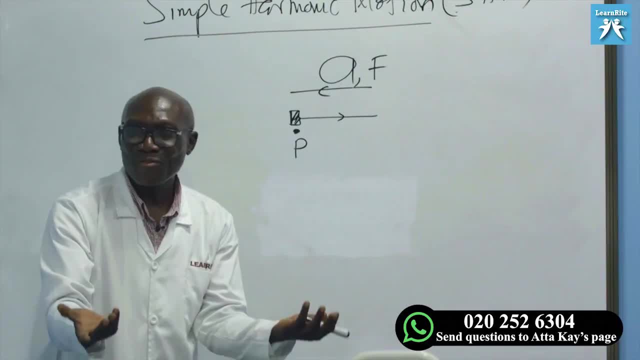 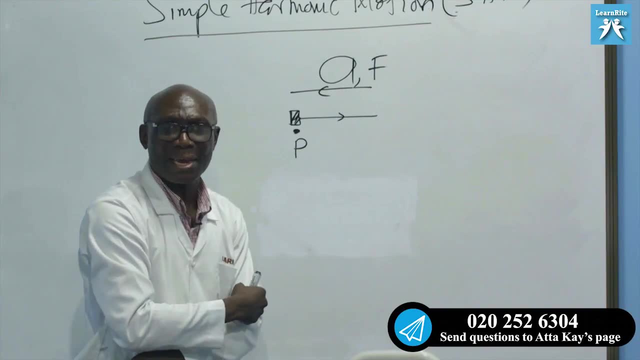 What will happen is this: The body cannot fight the force, So the body moves to a point and will have to follow the direction of the force. In other words, the body will come back. Now, when the body is coming back, they come back and then will bypass this point. 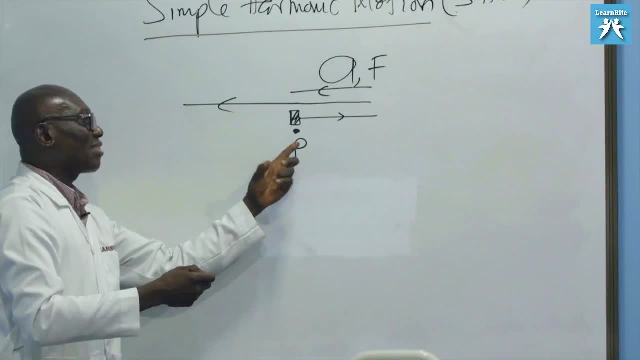 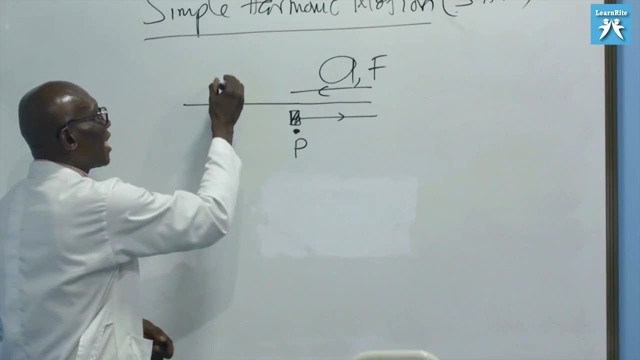 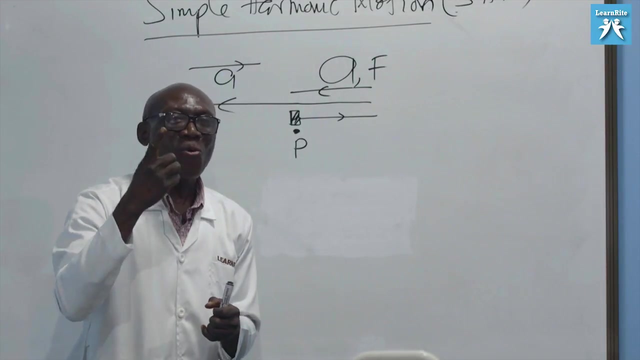 and go to the other side. And the moment it bypasses this point, this fixed point, and turns this direction, the acceleration will also turn, also to move in this direction. Do you know what is happening? The acceleration is always directed opposite to the direction. 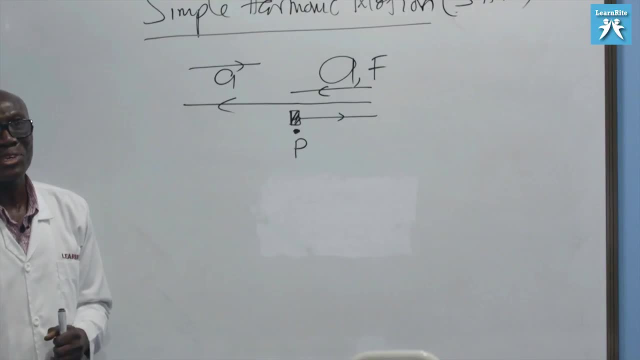 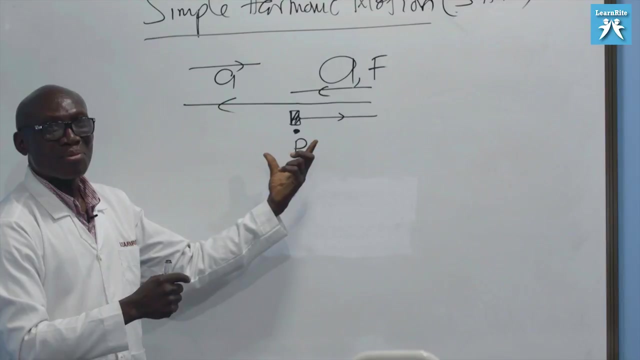 of motion Opposite to the direction of motion. So the acceleration is always directed toward this fixed point, no matter where you are, no matter where the position of the moving body. Not only that, Again, the acceleration possessed by the body is directly proportional. 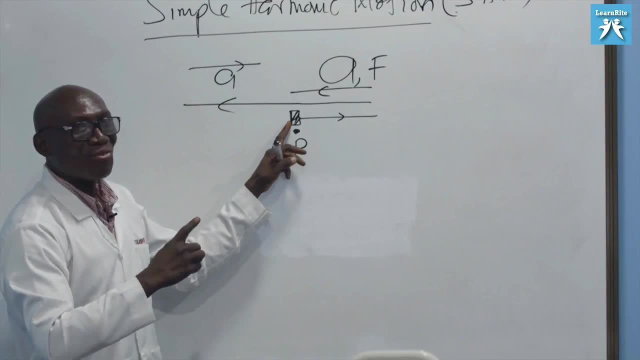 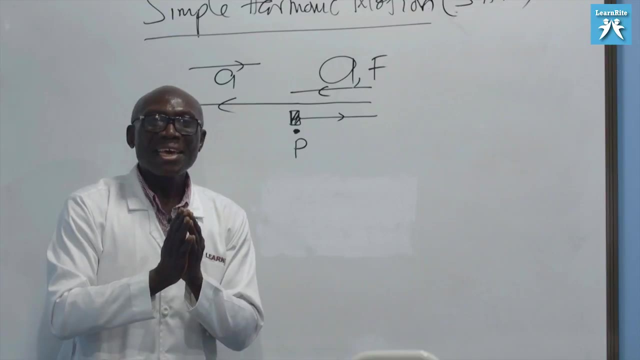 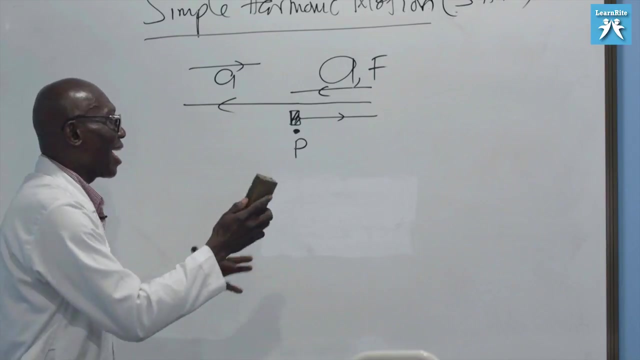 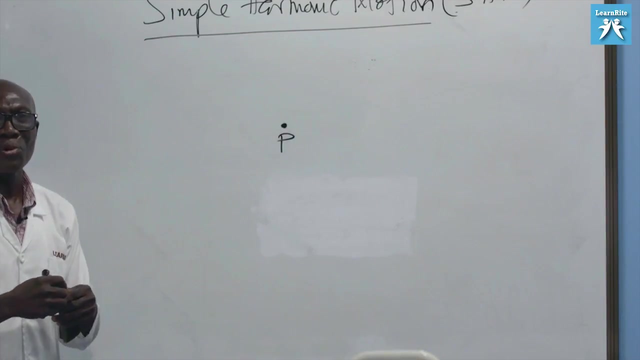 to the displacement of the body from the fixed point. Now put the two together and this is what we are calling simple harmonic motion. I will do just a brief explanation again and then we move on. I have this point T and I call this point the fixed point. 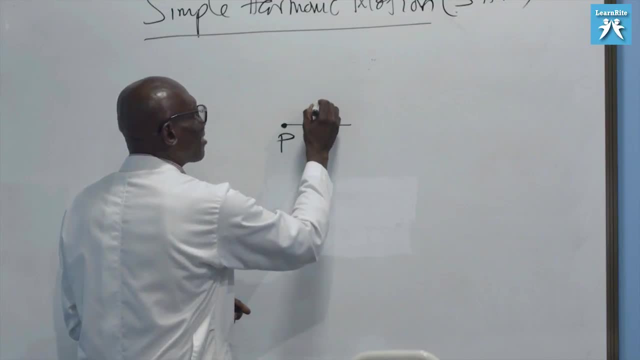 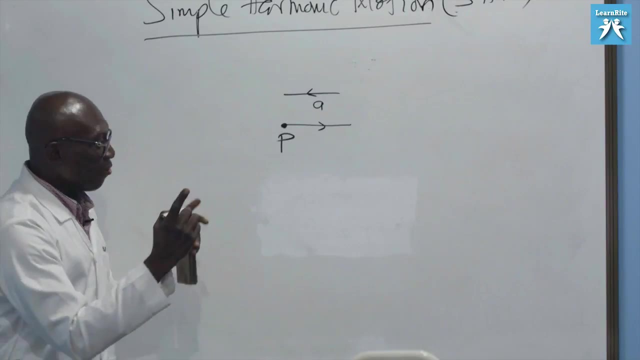 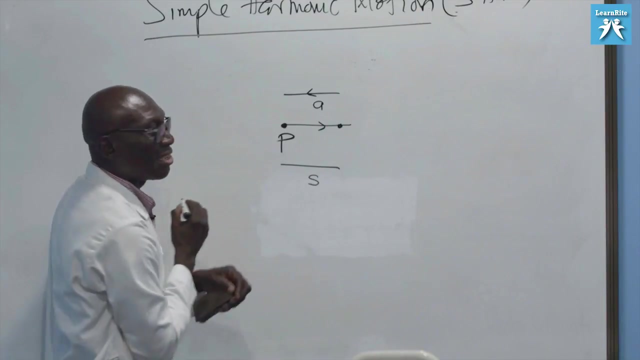 Now the body moves away from this fixed point, but its acceleration is directed to the direction of motion Opposite to it, towards the fixed point. Watch it: If the body has moved from here to there, this will be its displacement. I am using A to stand for the displacement. 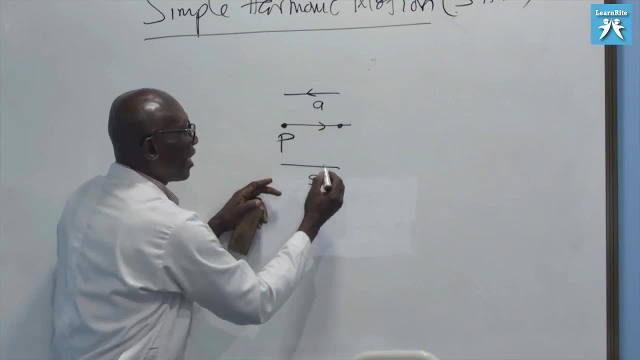 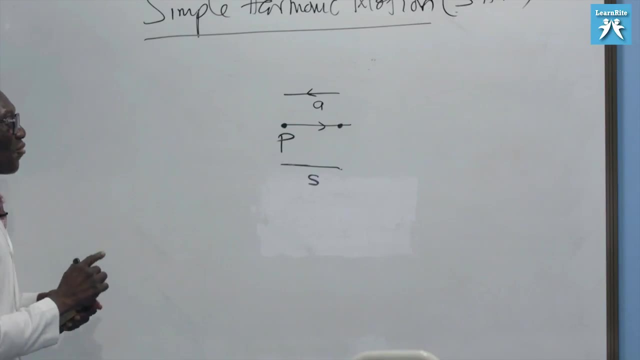 It has moved from A, which is the fixed point, to this point, somewhere there, and it has gone through a displacement S, A displacement S. Now, if the acceleration is always directed toward the fixed point, always directed toward the fixed point, Secondly, if the acceleration 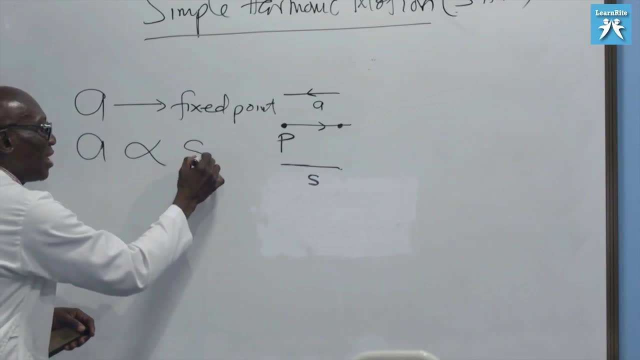 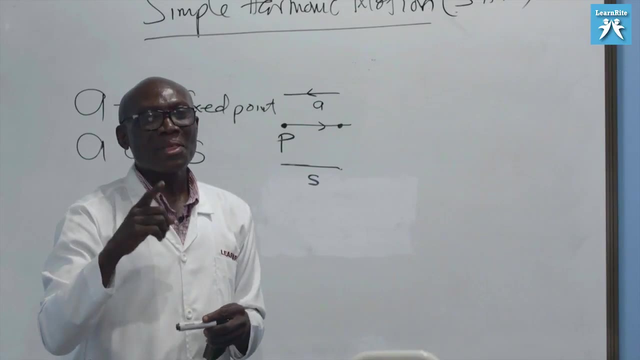 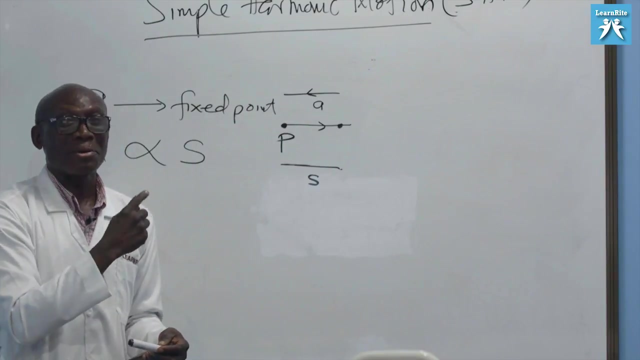 is directly proportional to the displacement from the fixed point. put the two together and we will call such a motion simple, harmonic motion. And in fact, if you check it very well, I said because the acceleration is always directed toward the fixed point. it is always 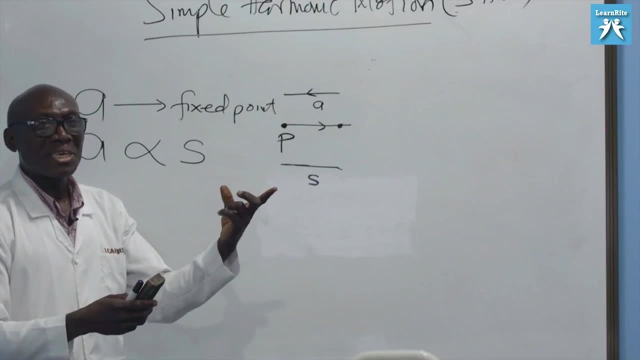 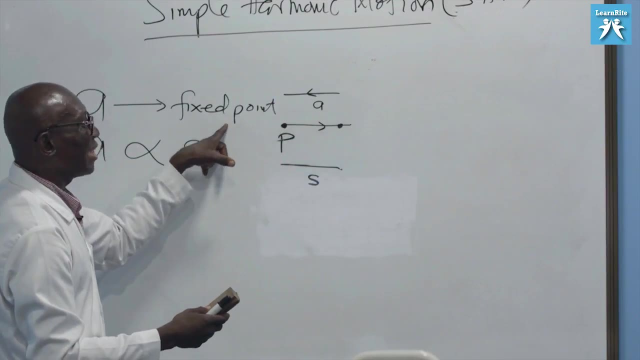 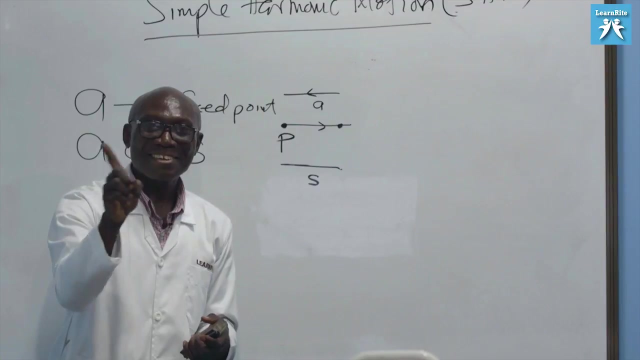 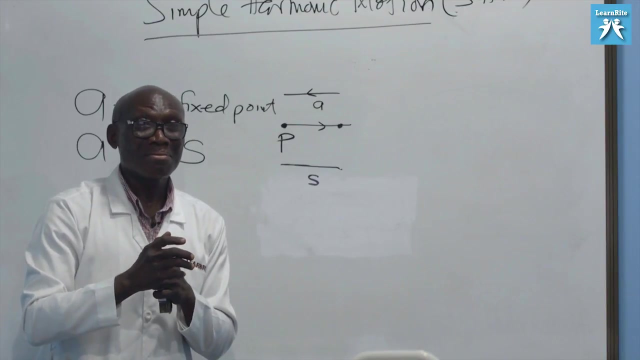 directed opposite to the direction of motion. The body is forced to come back. The body crosses this sign, this fixed point to this side. Acceleration will direct it back again and the body will end up doing this. So, in actual fact, simple, harmonic motion is an. 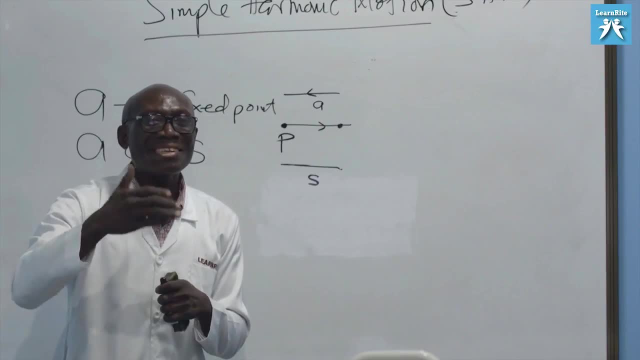 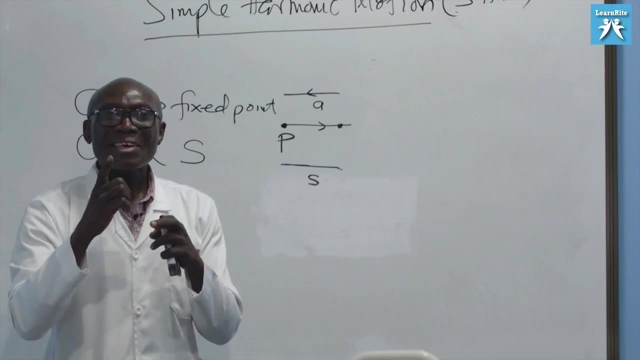 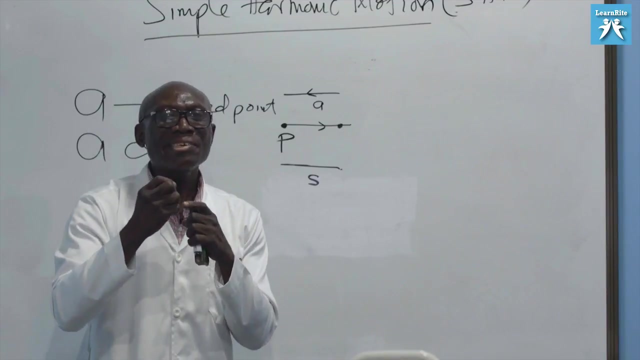 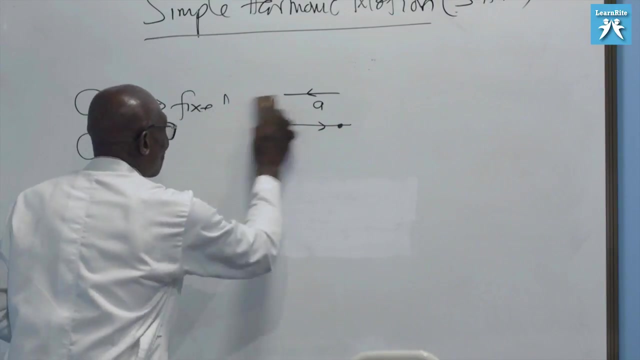 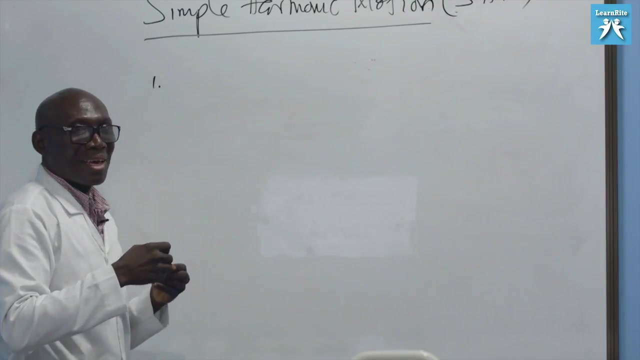 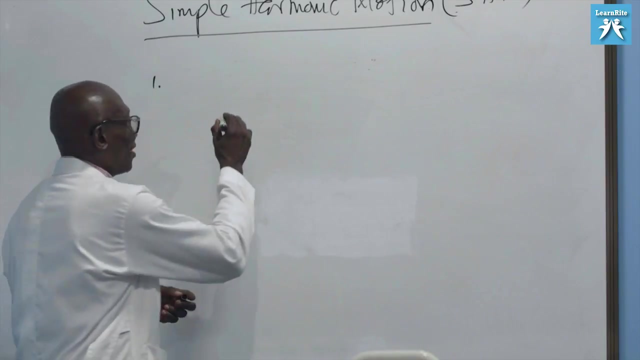 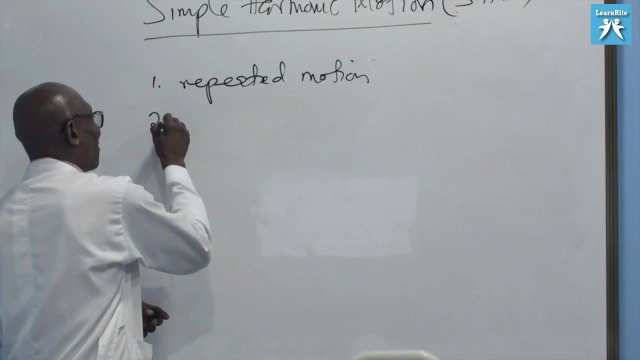 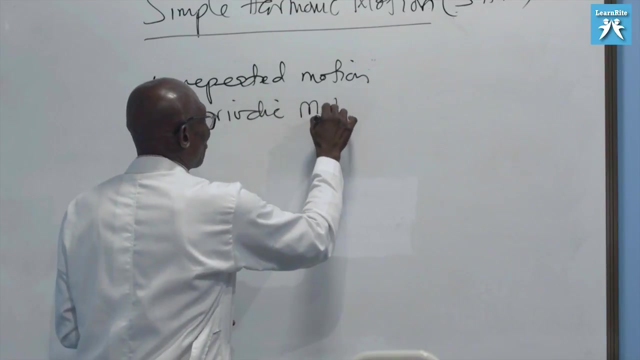 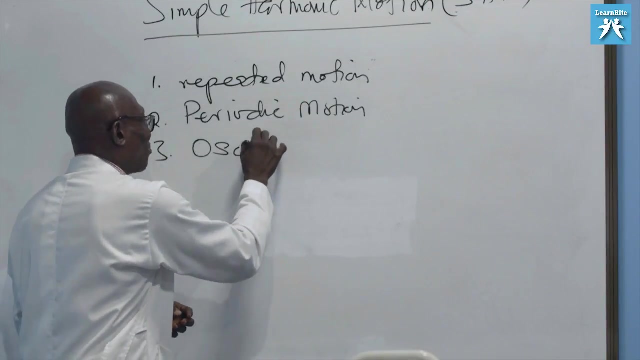 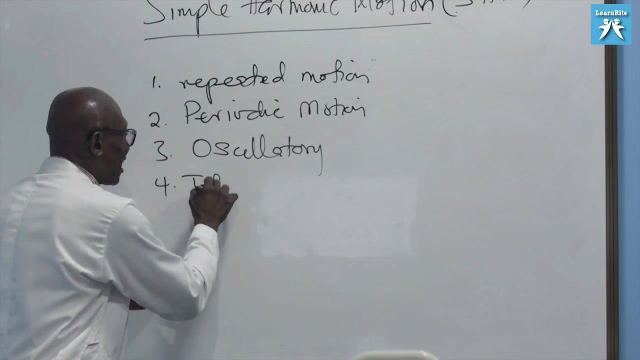 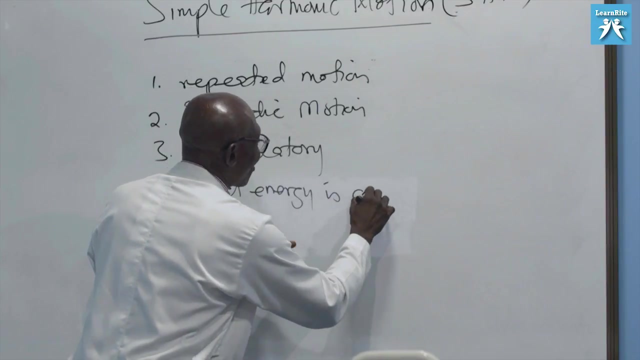 oscillatory motion, but with certain qualities. and I repeat, simple harmonic motion is an oscillatory motion with additional qualities or additional properties. and what are they? one SHM shows a repeated motion. it shows a repeated motion to SHM, shows a periodic motion. three: SHM shows oscillatory motion, for the total energy of SHM is constant, if I 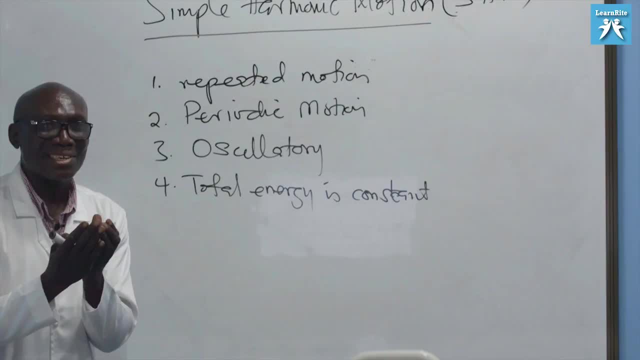 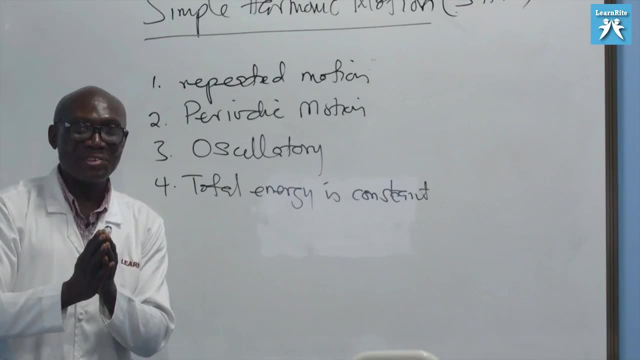 don't want to use the word constant. we simply say is conserved. when you conserve something, you are preserving. nothing is taken away, nothing is added to it, so it remains constant. again, the frequency. the frequency of the motion does not depend on the amplitude. the amplitude of the 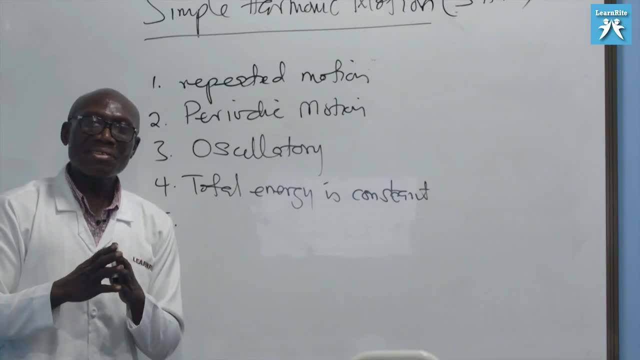 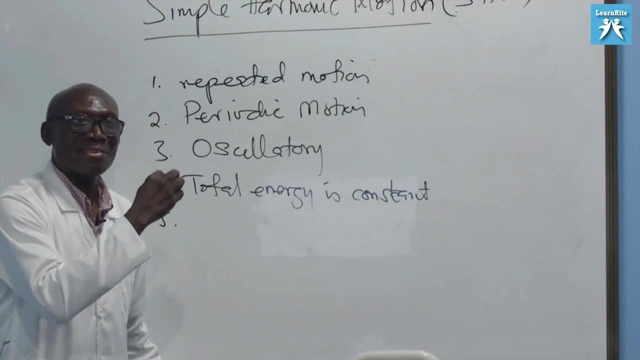 oscillation or the motion. students, I said we shall be dealing with this topic on its own. don't worry, we will see this and we shall talk about this into details. but what I want to say is this: when we are talking about simple harmonic motion, all these things are 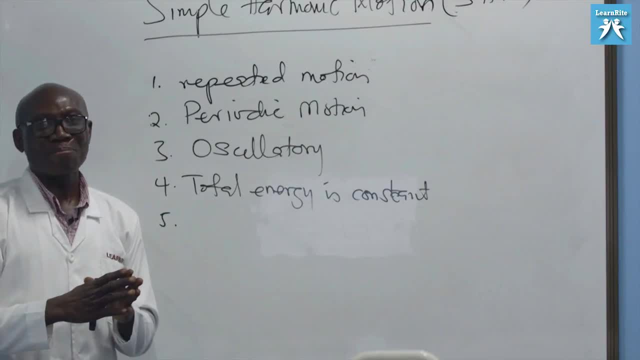 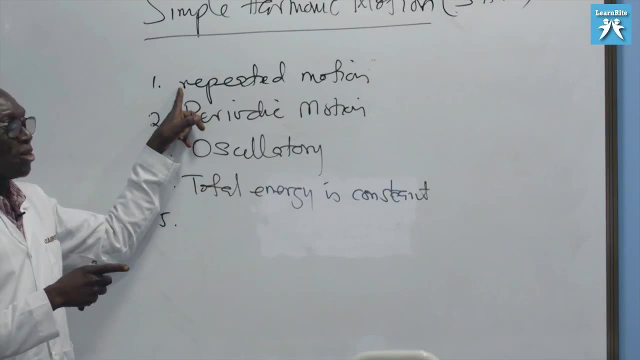 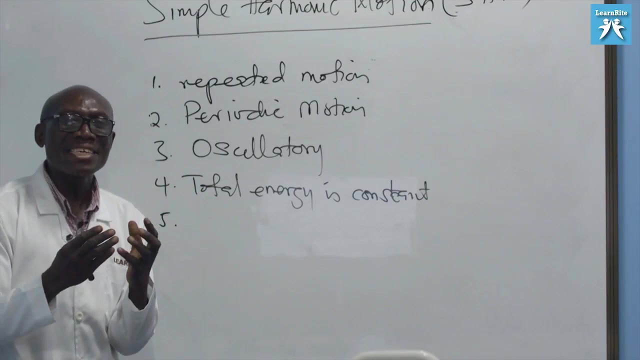 embedded in the simple harmonic motion. anytime a body is performing simple harmonic motion, you see the body showing repeated motion, you see it showing periodic motion, you see it showing oscillatory motion and you see the body having its total energy conserved. Conserve, Conserve. 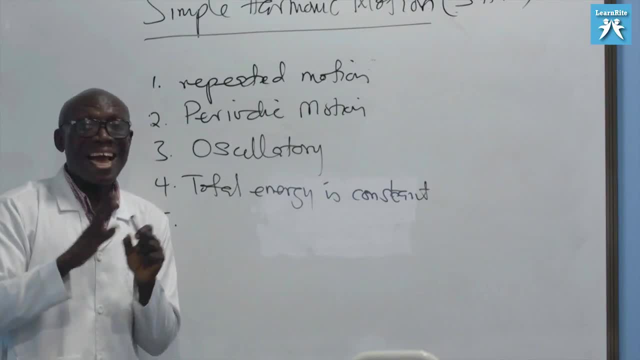 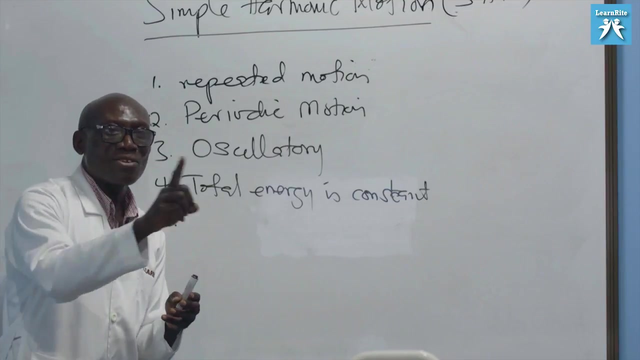 Conserve, Conserve. frequency of that motion, again, does not depend on the amplitude. so you see, as I said, if you are to give examples of simple harmonic motion, then you'll be given examples of motion that is to and fro, to and fro, to and fro. so let's look. 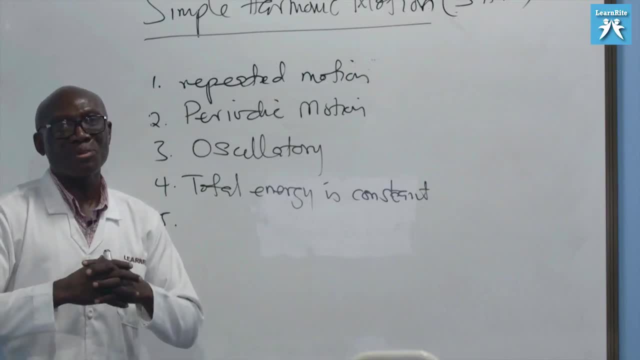 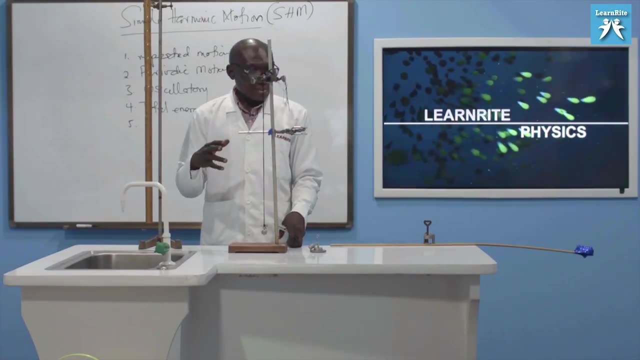 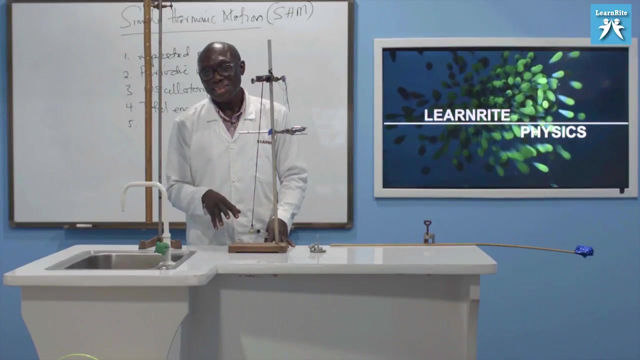 at the examples that we can give for simple harmonic motion. so dance with me. on the table are some of the few examples- and very important examples that we are going to give. they are important because these things you see here are the things that appear in your hands. 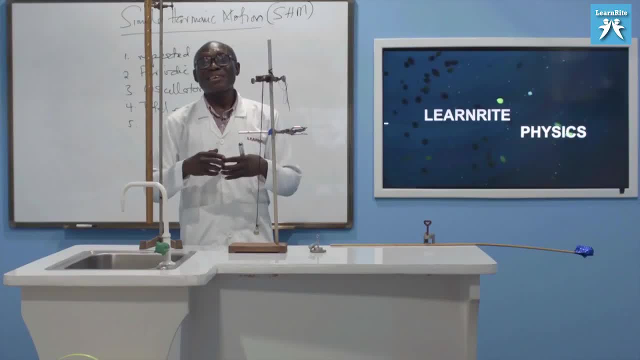 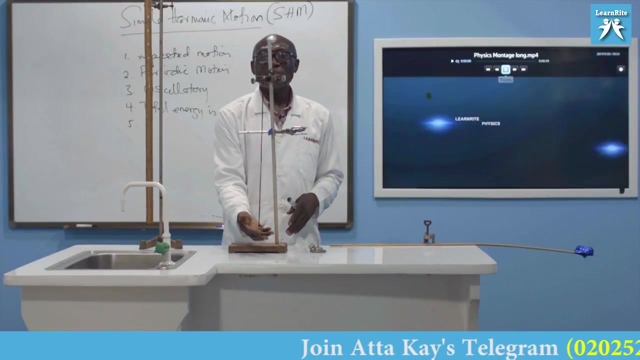 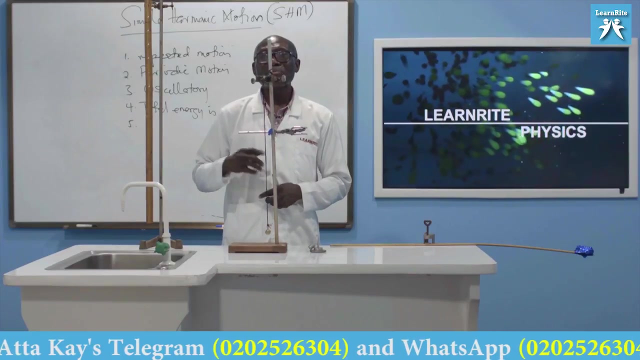 in fact, when we are talking about experiments on mechanics, most of them, most of them, are simple, simple harmonic motion experiment. and we have these examples now. the first one has to do with a simple pendulum, and you can see it, simple pendulum. now let's see how it performs simple harmonic motion and, as I said, simple harmonic. 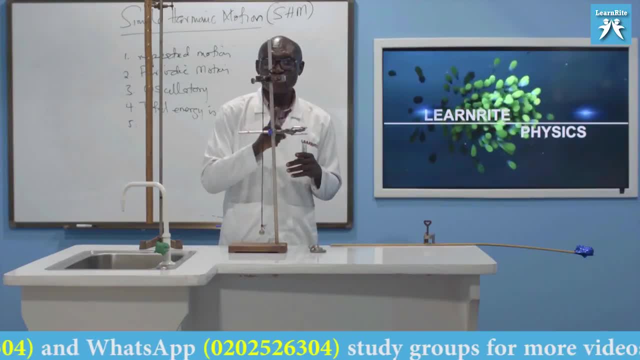 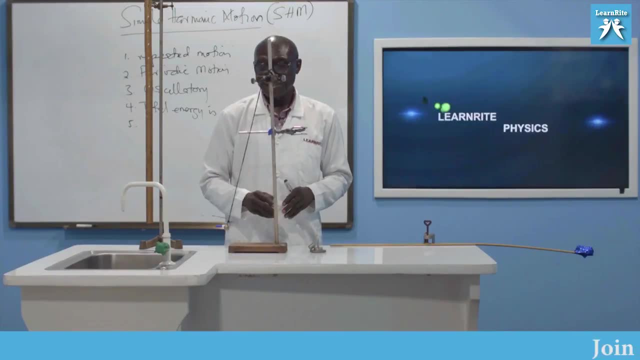 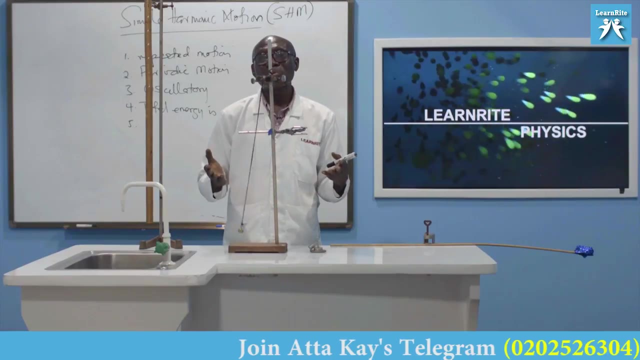 motion in actual fact shows to and fro, to and fro through. So what we do is to swing it and then you leave it. You just place it through a small angle and you leave it, And that is it. It performs simple, harmonic motion, Alright. 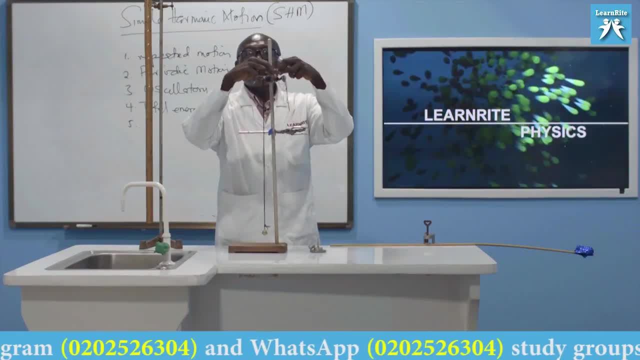 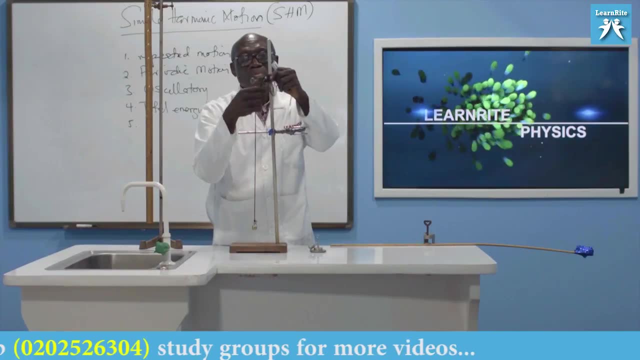 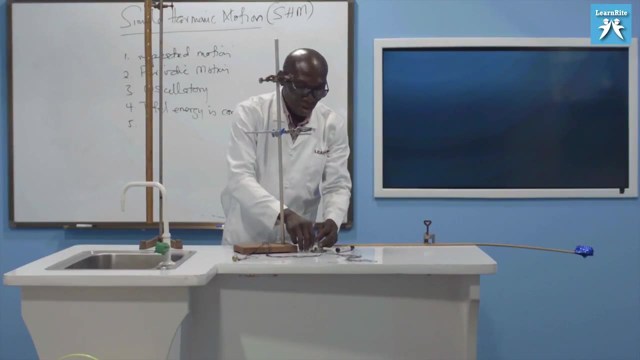 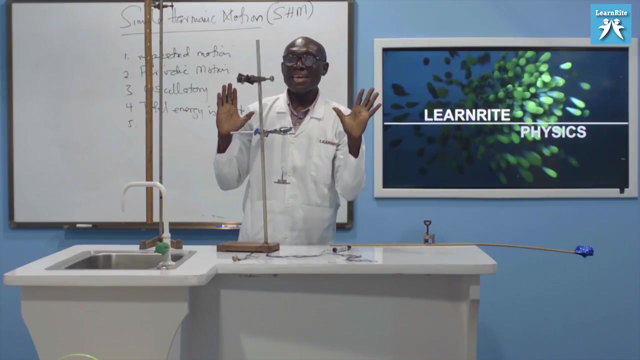 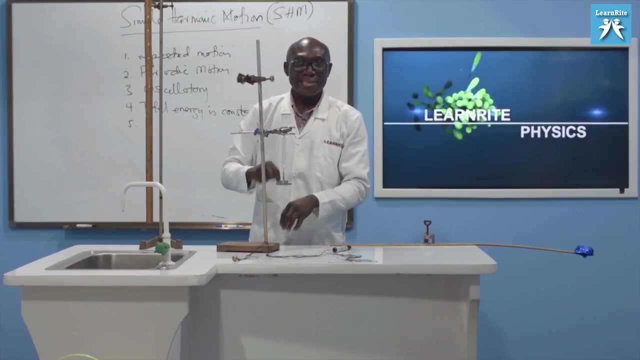 The next one has to do with the spring- elastic spring. I will take the pendulum off and then I will mount this spring on this tan. can you see that This is the spring? and the spring has been weighted, or it has been loaded? It means something has been hanged on it Now. 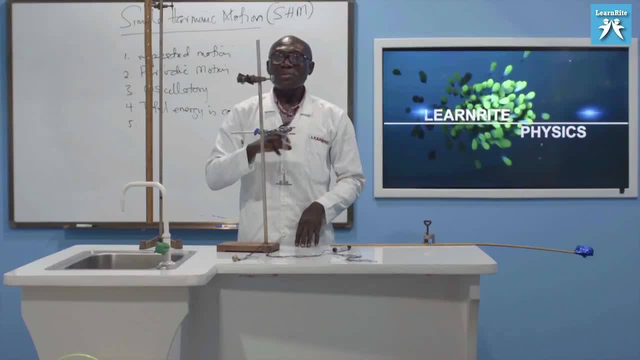 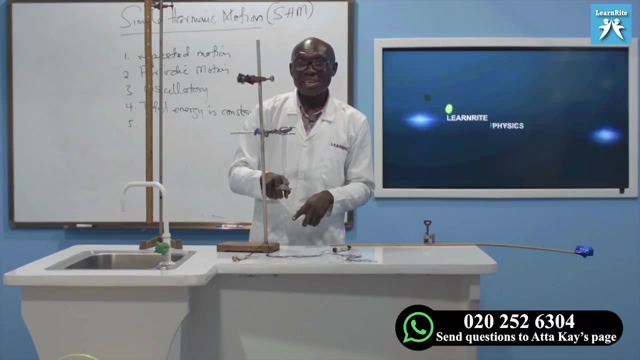 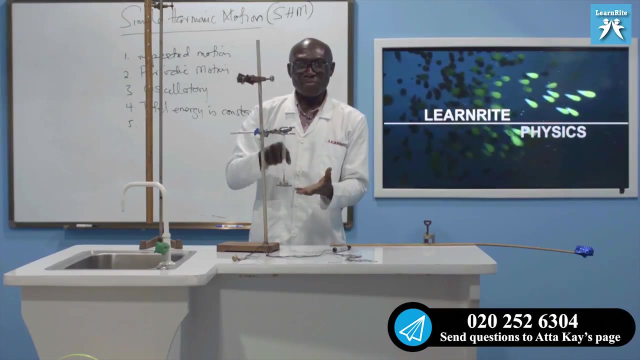 we are going to cause this spring to perform simple harmonic motion. So what I will do is to displace this spring downwards a bit and leave it, And that is it. Please, if you should displace this one through a large distance, something will happen and I will. 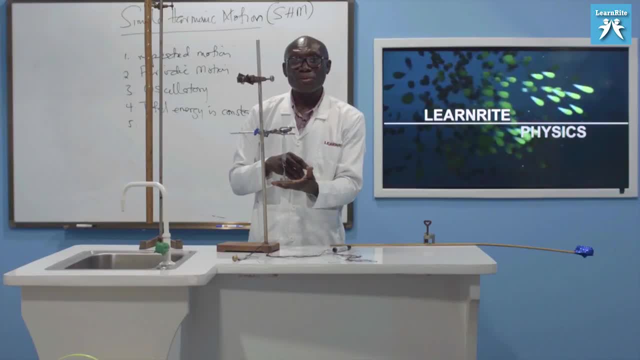 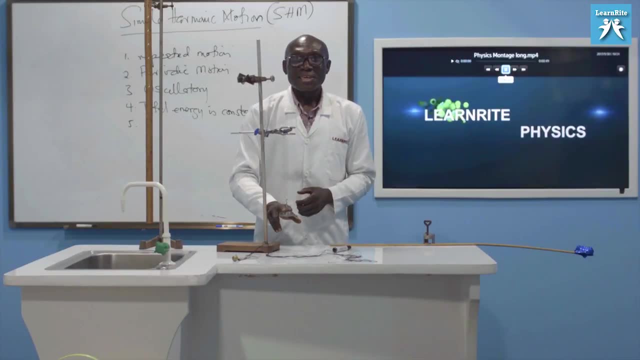 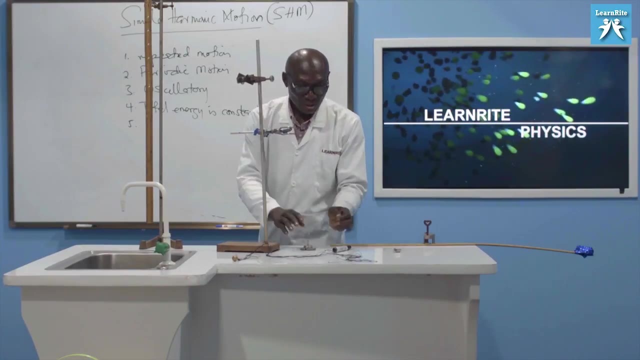 show you, And that is why it is always advisable to displace the load through a small distance, and I'm going to do that for you to see. Now, watch it, I'm even afraid. Do you see what is happening? All right, All right. So to avoid this, it is always said that you should. 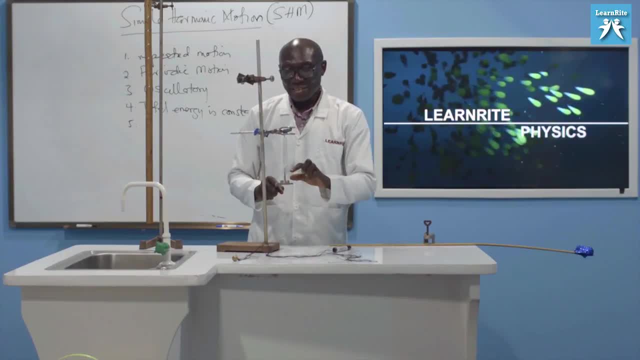 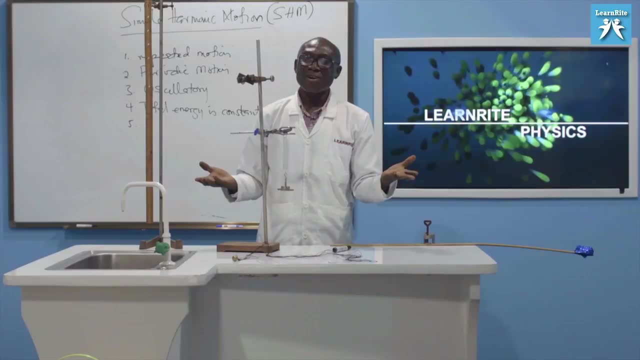 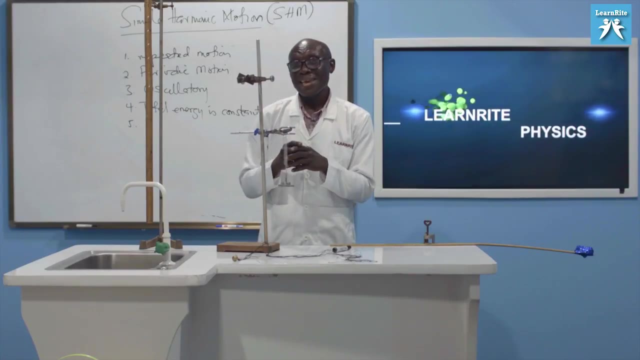 displace the load, And that is what we expect you to do- That displace it through a small angle, Just a small distance. Displace it and leave it. See how wonderful and how beautiful the oscillation is. Take note of this. Don't worry, We shall be doing this again under 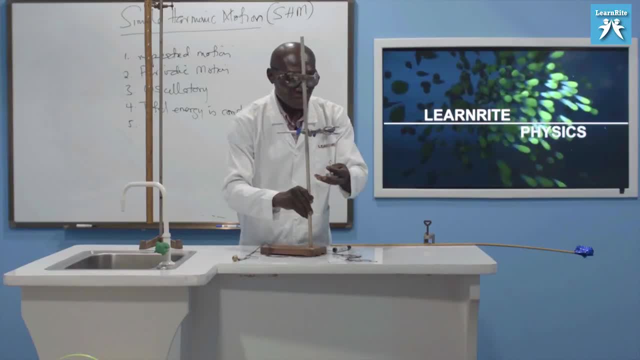 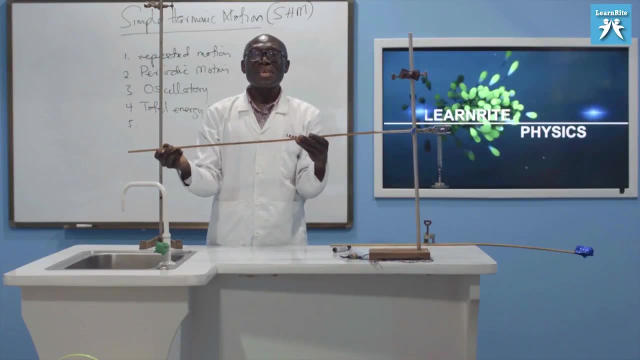 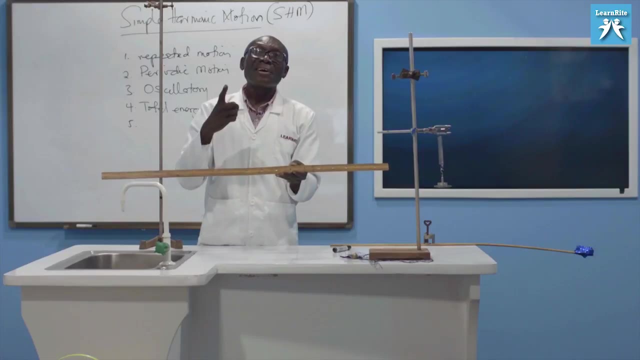 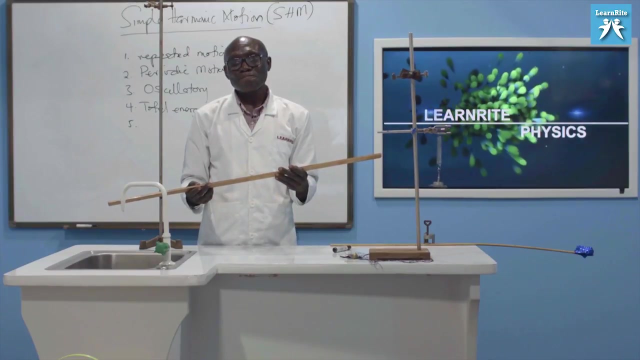 the topic SHM. Then we also have what we call a compound pendulum. We call this one a compound pendulum. This is a meter rule with holes drilled along it, And most of the time the holes are five centimeters apart along the entire length of the ruler. So what you do is to suspend. 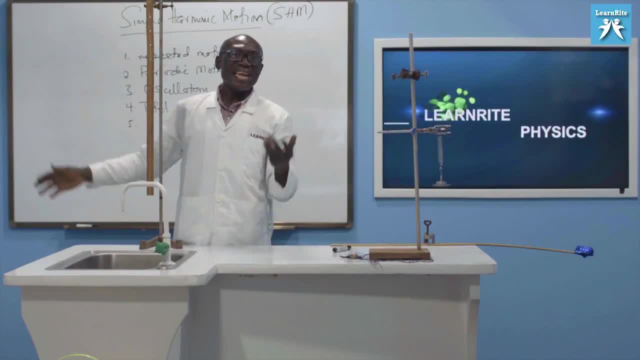 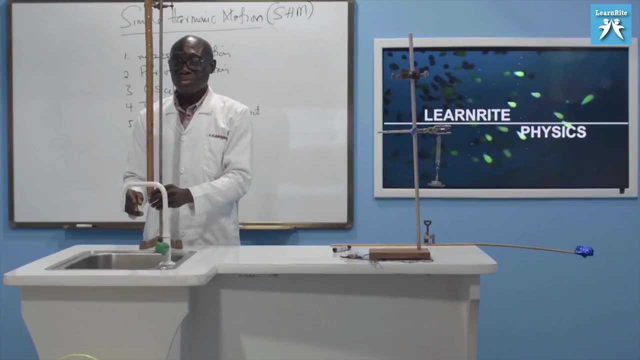 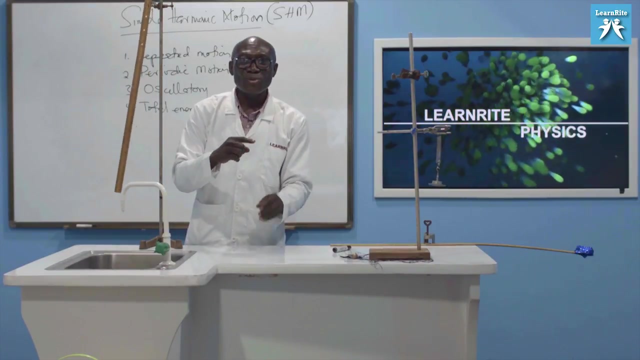 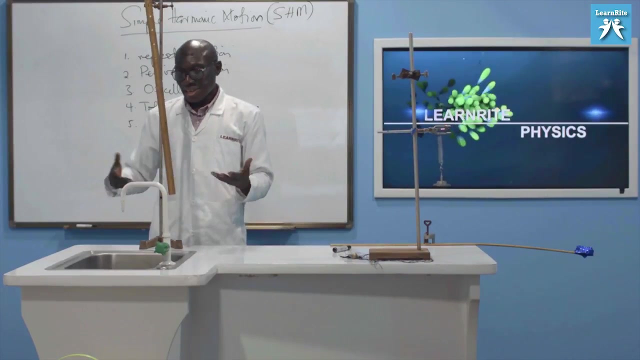 this compound pendulum through any of the holes. And here we are. Now I'm going to displace this one through a small angle and leave it, And it swings, Please. The displacement is always through a small angle or through a small distance, Just a small distance or small angle, And it is swinging. This is what we 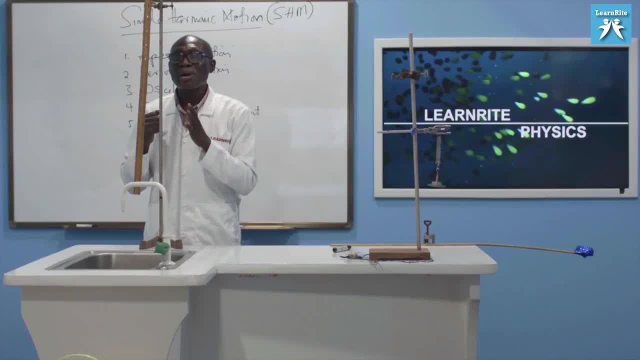 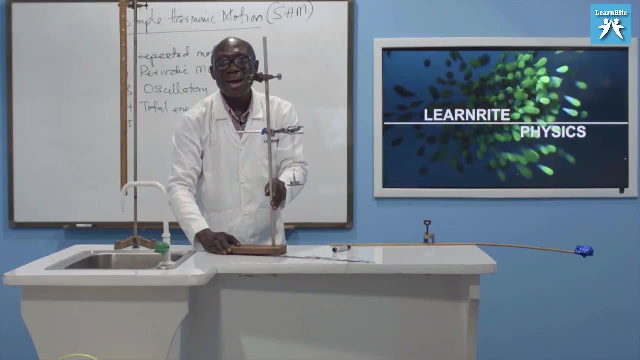 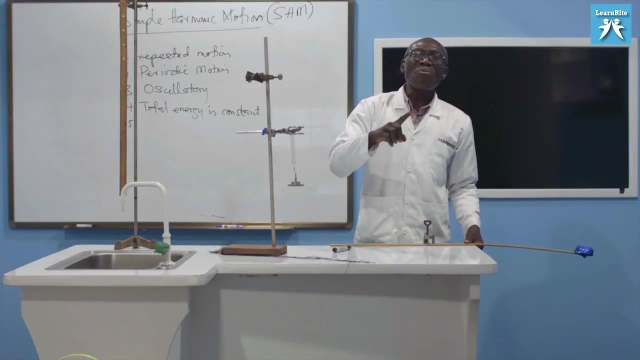 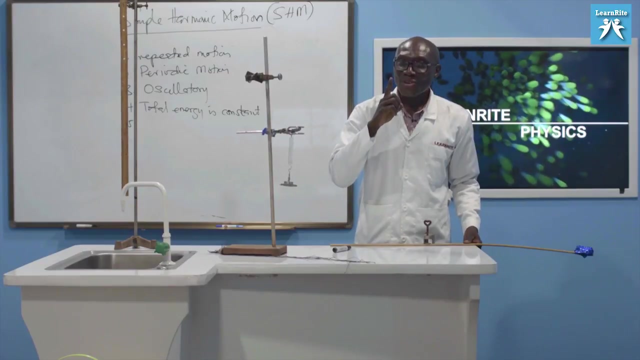 call the compound pendulum, Compound pendulum. We have been finished. We have what we call the cantilever Cantilever. And now we are taking our time to show you all this because almost all the practicals that, as I said, you do on mechanics, most of them are on simple. 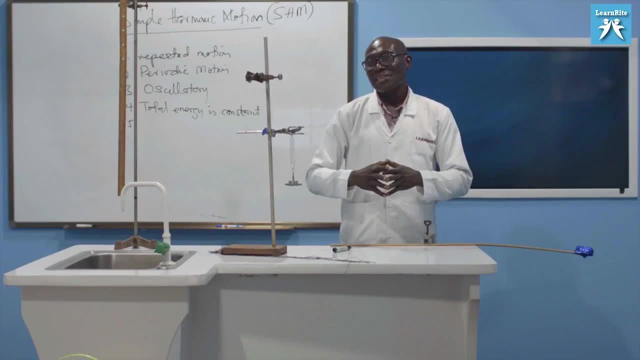 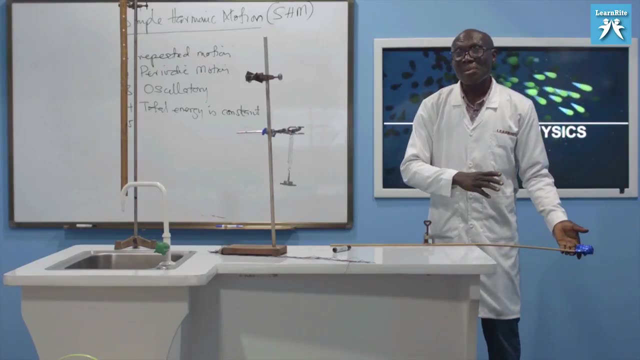 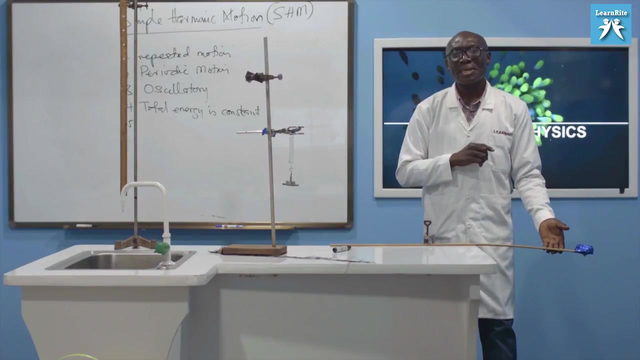 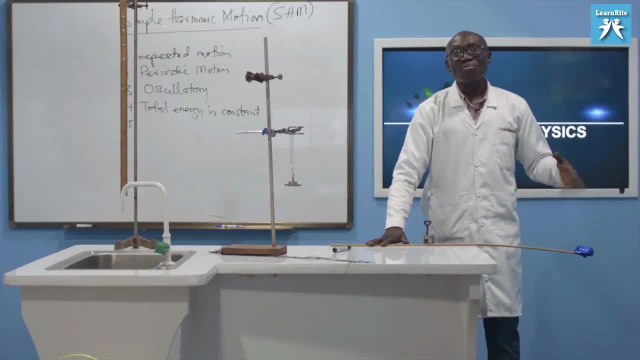 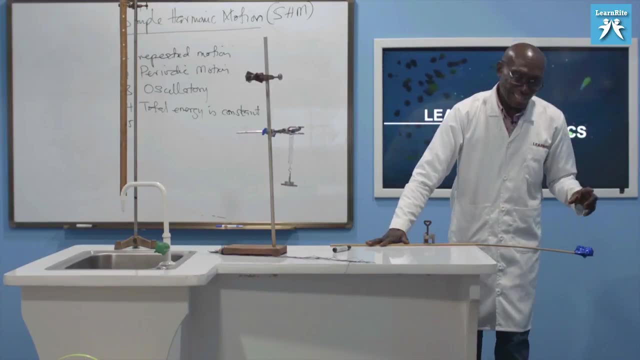 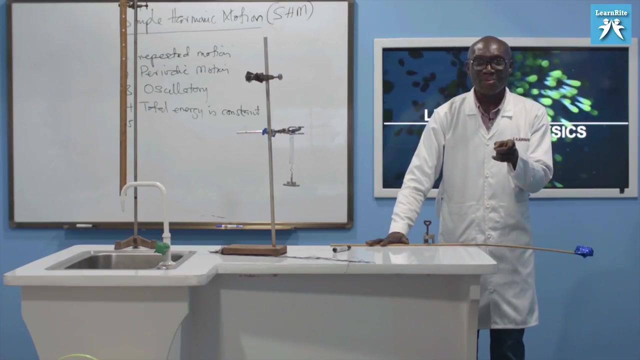 to do it. I'm going to show you how to do it. It's on the bench And the other session protrudes, Portrudes out of the bench. Now, normally it is weighted, In other words, a load is hung here so that it will slow down the motion. You will be counting and should. 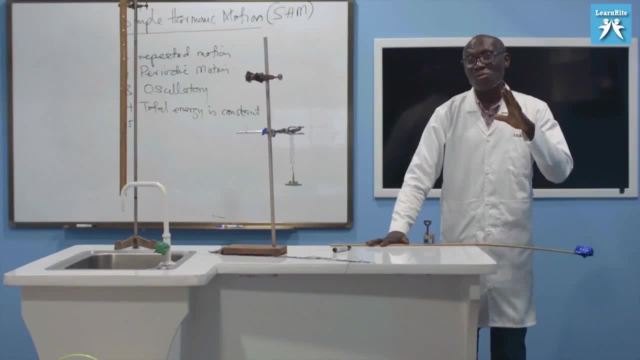 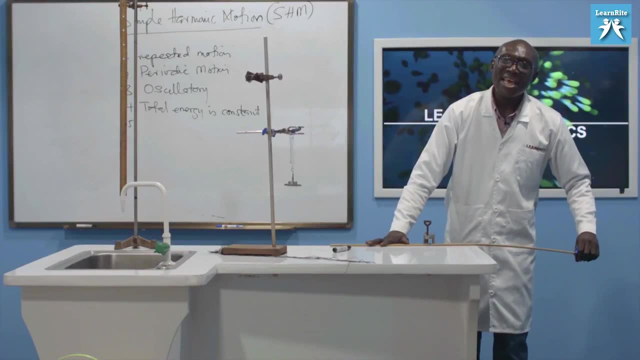 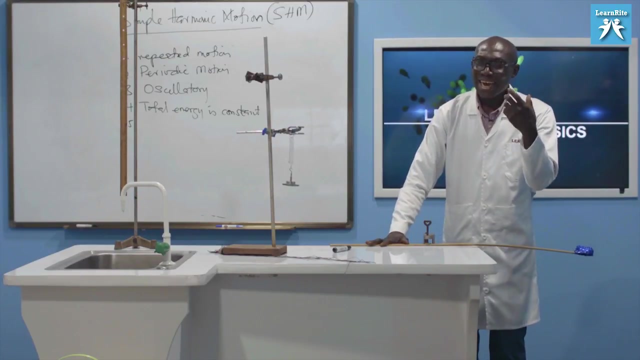 be able to count how many oscillations. So we must be able to slow the motion down. So most of the time the question will ask you to put something here, a load here, and they will specify the mass that we are supposed to put there. even when they don't ask you to do that, you can still. 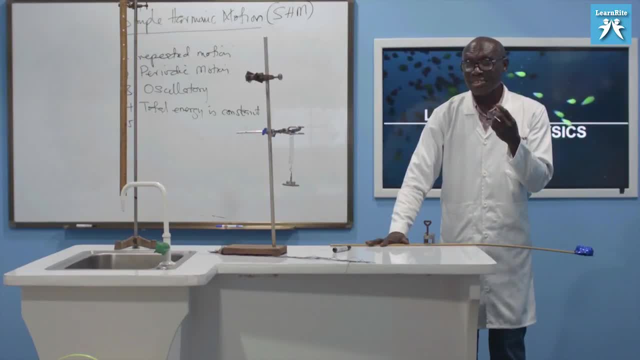 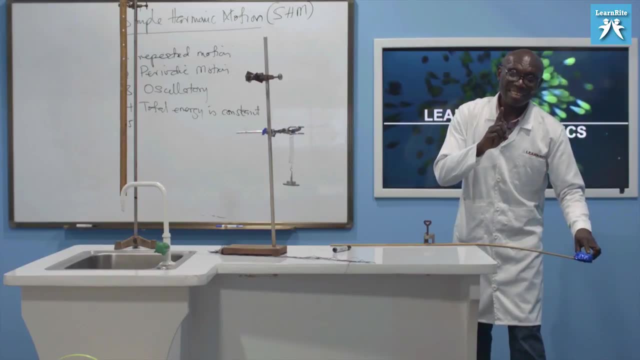 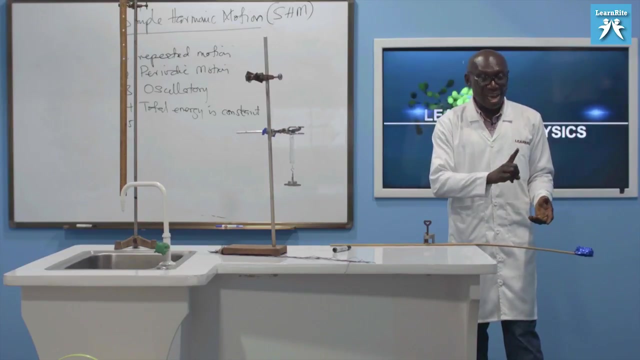 count. you can take only that. you do that with some difficulty. now let's see what happens. I'm going to display this one down slightly, slightly and I will leave it, and then you can see it. you can see that, and that is to and fro, to and fro. 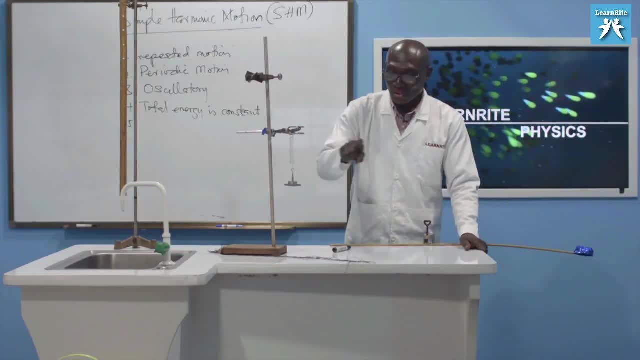 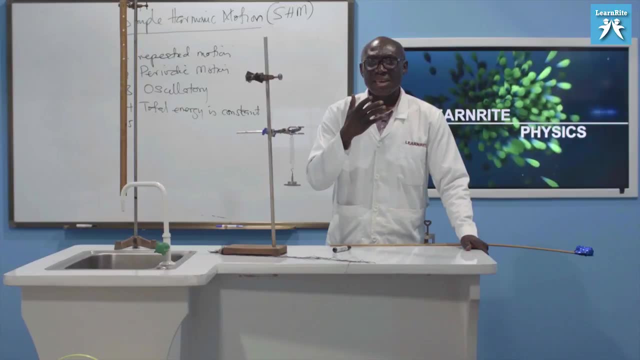 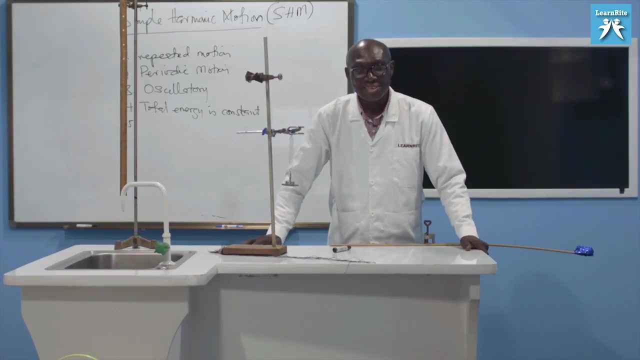 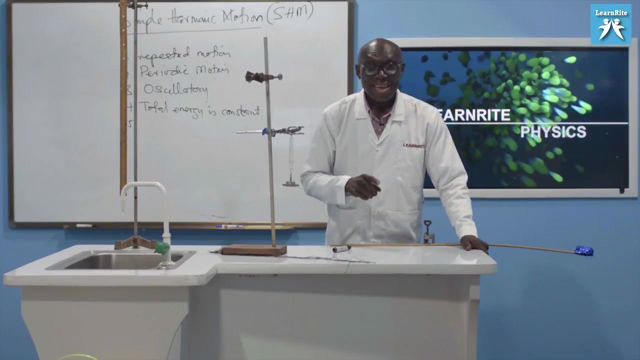 you know what the to and fro can be horizontal and it can be vertical. that is why when we're in school- and I don't know whether you are doing this disease any time- somebody is doing off in a classroom, we always say that the head is performing SHM, somebody who is doing snuff- it's always like that and that head. 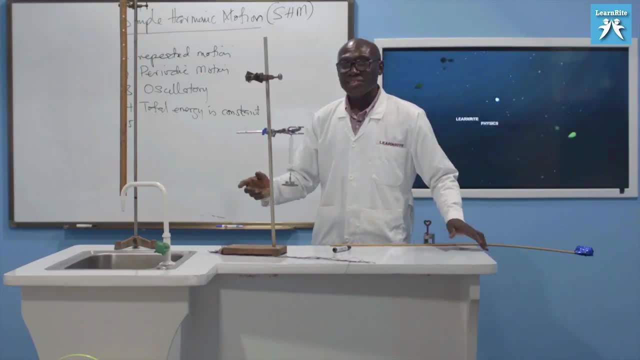 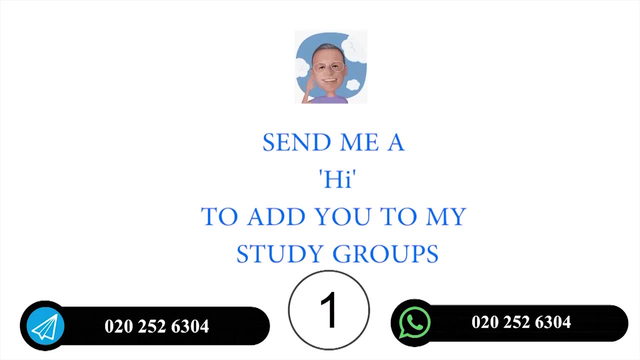 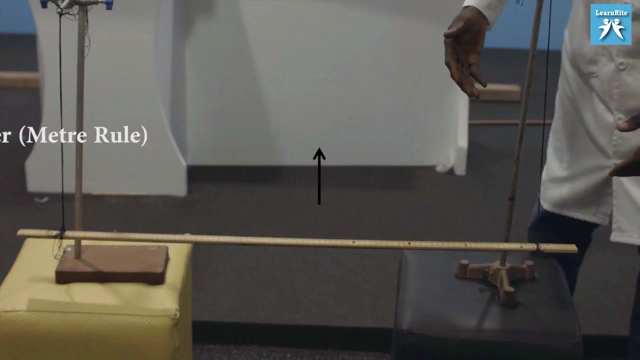 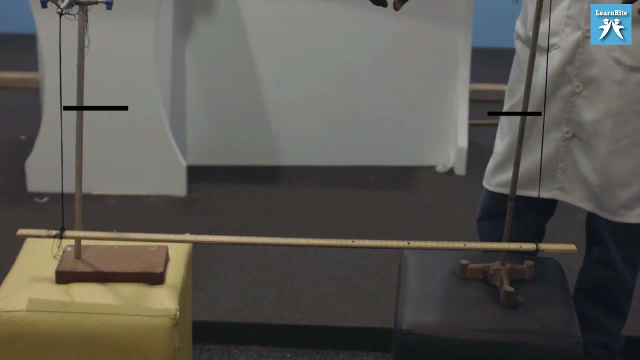 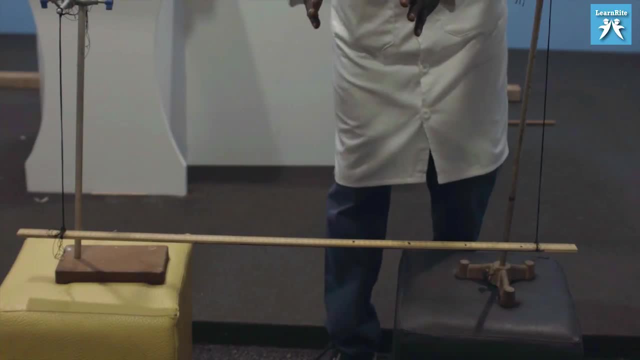 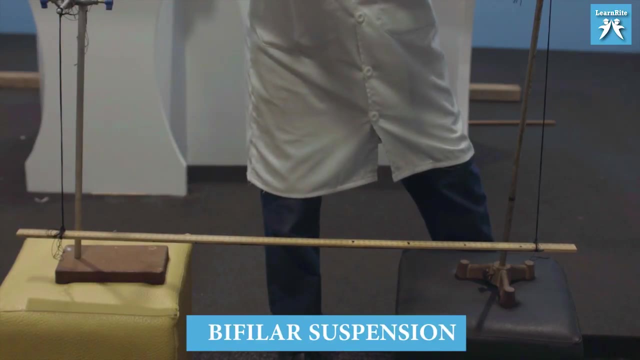 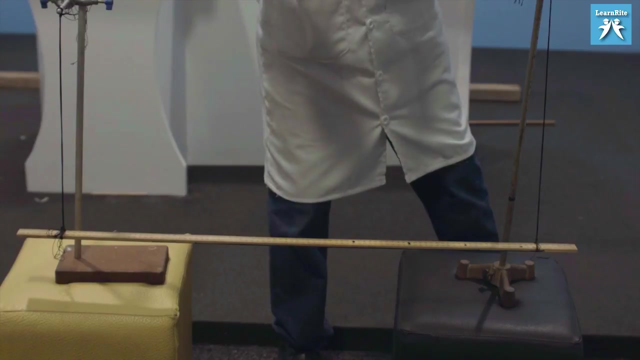 so here we are, a ruler mounted horizontally on two strings, and these two strings are held by two retostans. this arrangement is simply called a by filler suspension. now we are going to. this arrangement is simply called a by filler suspension. now we are going to cause this suspension to perform SHM. and watch me carefully, watch my hand. 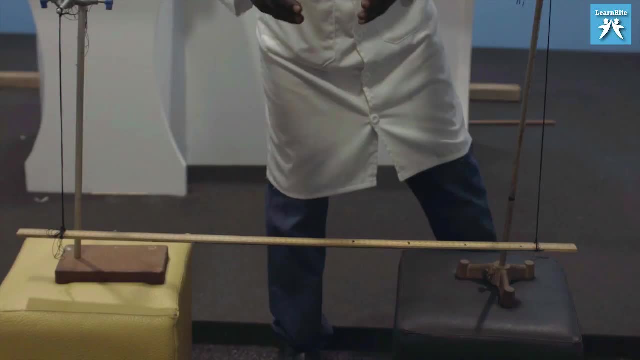 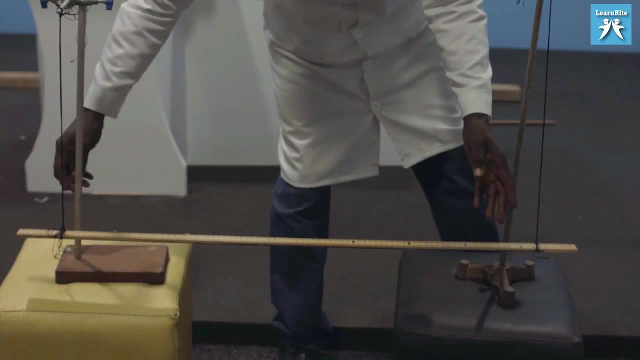 cause this suspension to perform SHM. and watch me carefully, watch my hand carefully, the way I'm going to set this to be in motion and go strictly by that carefully. the way I'm going to set this to be in motion and go strictly by that carefully. the way I'm going to set this to be in motion and go strictly by that. I'm going to hold the two and 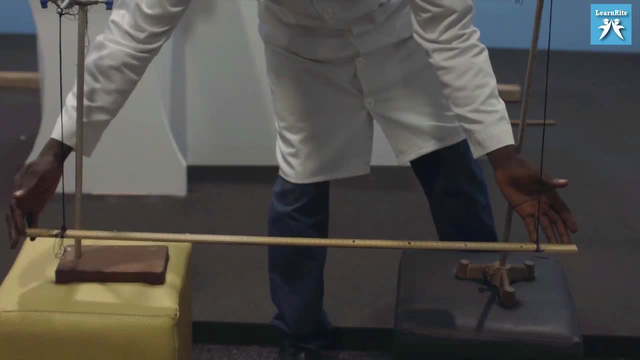 I'm going to hold the two, and I'm going to hold the two and ends- two ends, and I will displace them in ends- two ends. and I will displace them in ends- two ends, and I will displace them in opposite directions. so I'm going to do 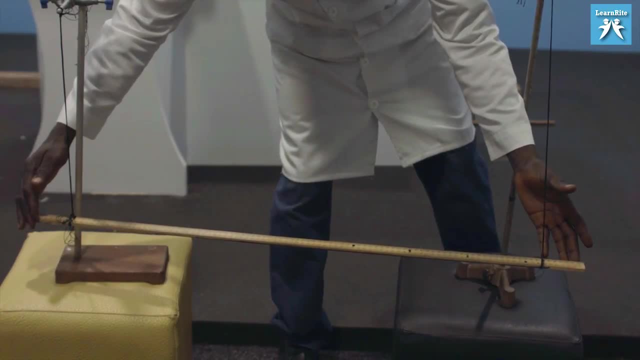 opposite directions. so I'm going to do opposite directions. so I'm going to do this in opposite directions and I will this in opposite directions and I will this in opposite directions and I will leave it and it swings. it swings like: leave it and it swings. it swings like. 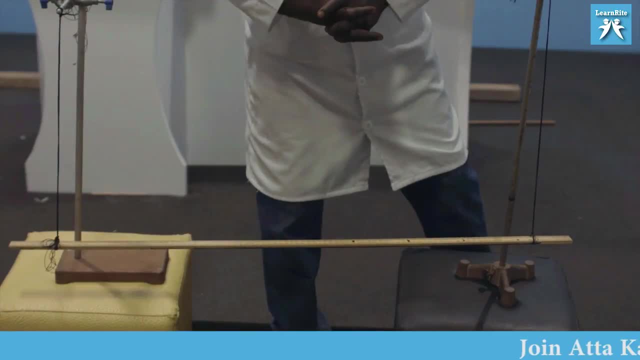 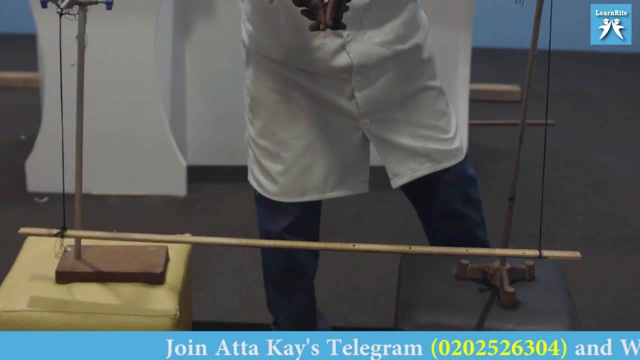 leave it and it swings. it swings like that. this is all about by filler, that this is all about by filler, that this is all about by filler. suspension. but I want to caution you here. suspension. but I want to caution you here. suspension. but I want to caution you here. I've seen students doing this and that. 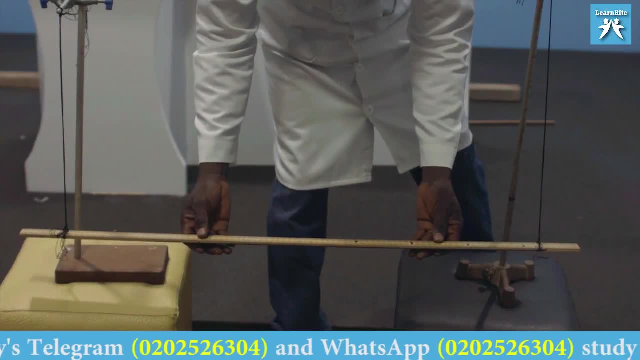 I've seen students doing this and that I've seen students doing this, and that is extremely dangerous, is extremely dangerous, is extremely dangerous. this is what they do. they swing the whole. this is what they do. they swing the whole. this is what they do. they swing the whole meter rule and they leave it, are you? 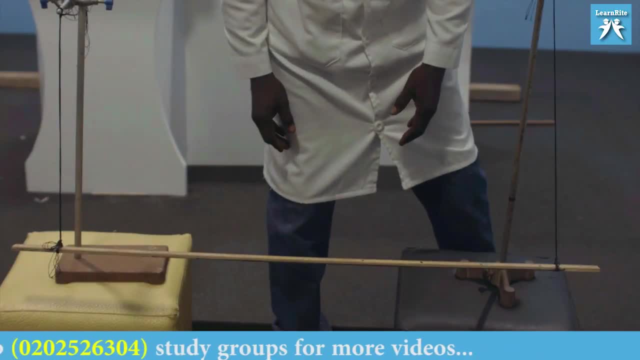 meter rule and they leave it? are you meter rule and they leave it? are you watching me and they leave it? and this watching me and they leave it. and this watching me and they leave it. and this is what you see happening. this is wrong. is what you see happening. this is wrong. 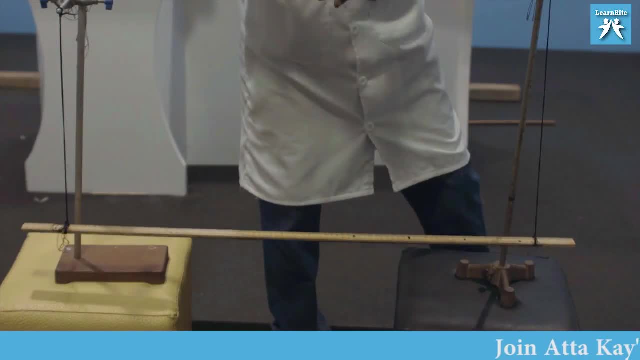 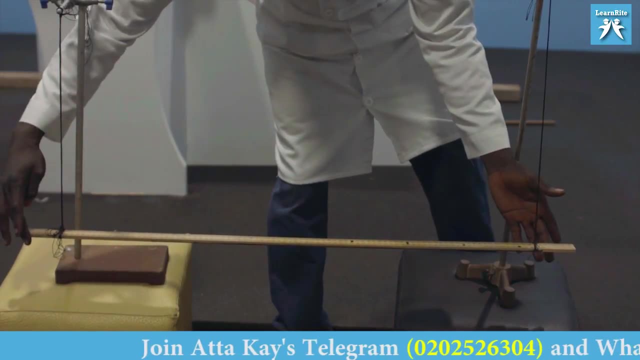 is what you see happening. this is wrong. this is wrong. this is not by filler. this is wrong. this is not by filler. this is wrong. this is not by filler. suspension: what you have to do is to suspension. what you have to do is to suspension. what you have to do is to displace the two ends in opposite. 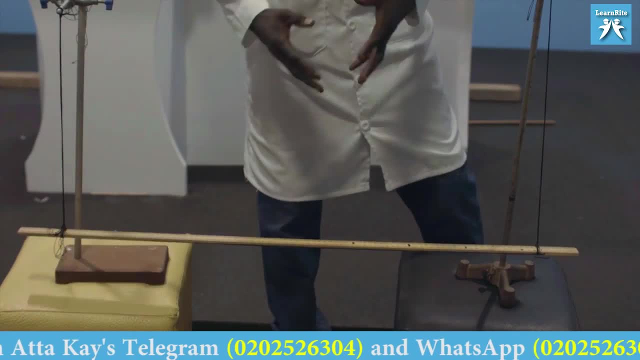 displace the two ends in opposite, displace the two ends in opposite directions, and then you leave it to directions, and then you leave it to directions, and then you leave it to the way you set the by filler suspension, to the way you set the by filler suspension to. 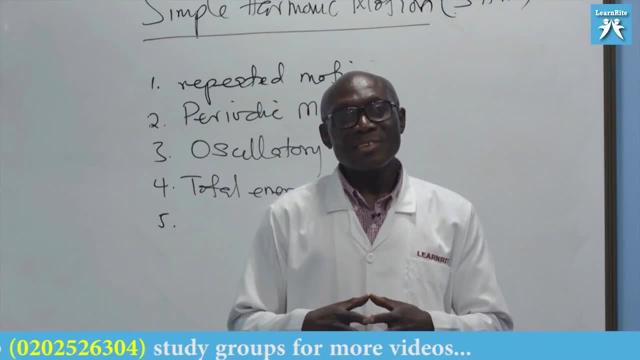 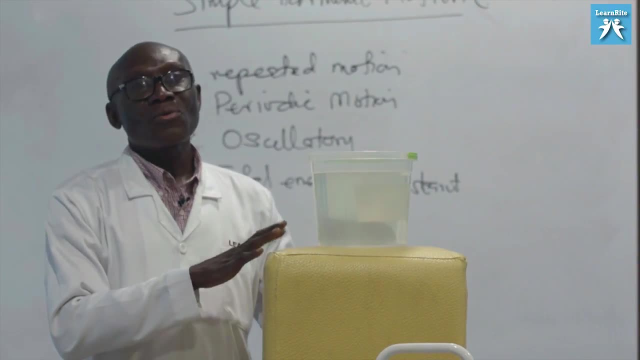 the way you set the by filler suspension to swing. I've cautioned you. let's look at swing. I've cautioned you. let's look at swing. I've cautioned you. let's look at the next example. this is the last. the next example. this is the last. the next example. this is the last example that we want to demonstrate in. 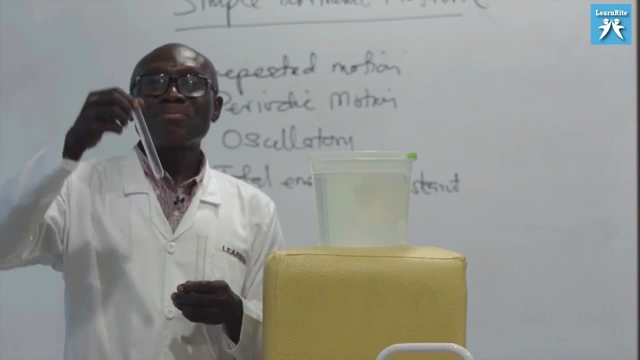 example that we want to demonstrate in example that we want to demonstrate in this studio. I have a test tube- an empty this studio. I have a test tube- an empty this studio. I have a test tube, an empty test tube. I want this test tube to stand. test tube, I want this test tube to stand. 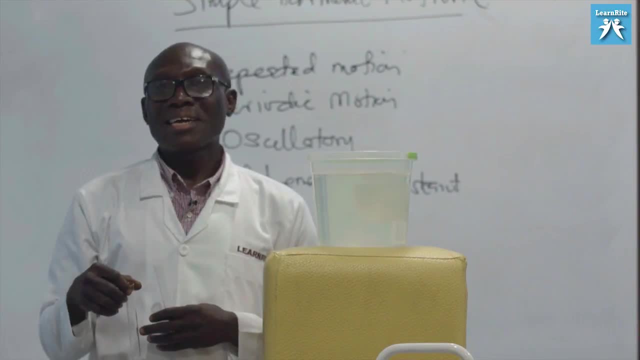 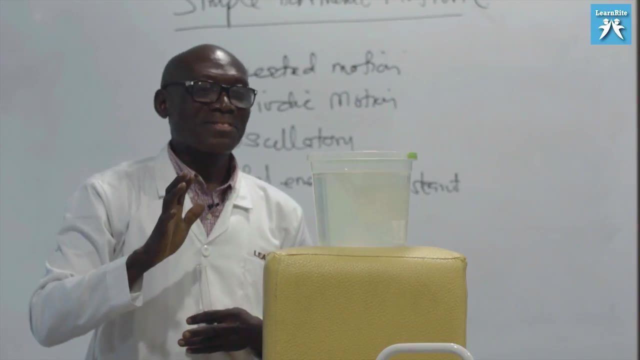 test tube. I want this test tube to stand upright in this water, but watch it. an upright in this water, but watch it. an upright in this water, but watch it. an empty test tube, empty test tube, empty test tube. if I leave it, it falls, it falls and 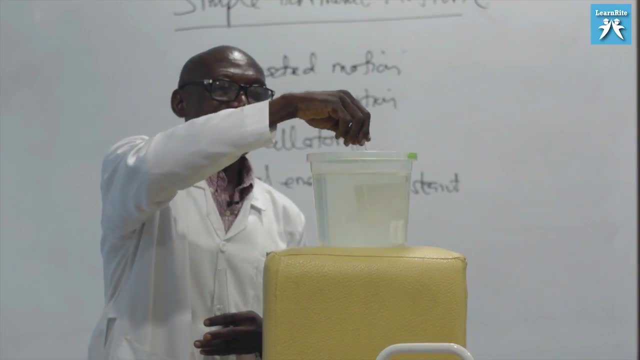 if I leave it, it falls, it falls. and if I leave it, it falls, it falls. and what I guess into it now, if I want to what I guess into it now, if I want to what I guess into it now, if I want to avoid the test you falling, what I will? 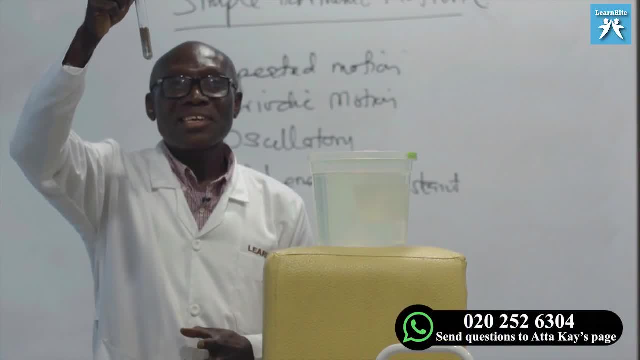 avoid the test you falling. what I will avoid- the test you falling, what I will do is to put something in the test you do is to put something in the test you do is to put something in the test you. and when you do that, it is said that the 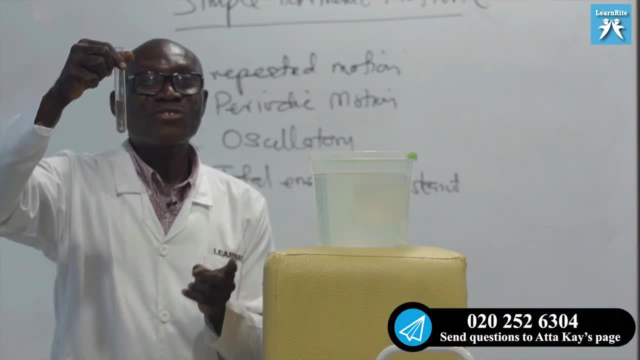 and when you do that, it is said that the and when you do that, it is said that the test tube is weighted. the test tube is, test tube is weighted, the test tube is test tube is weighted, the test tube is weighted or the test tube is loaded. so 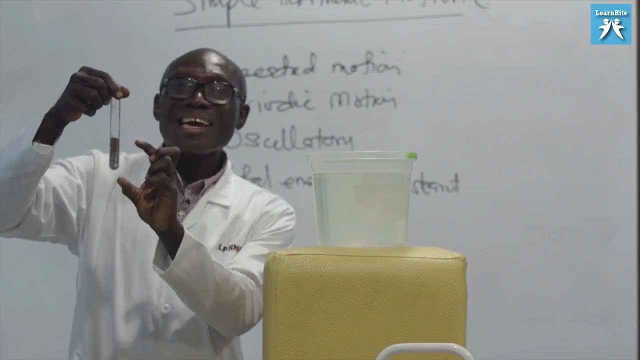 weighted, or the test tube is loaded, so weighted, or the test tube is loaded, so when you load a test, you and you load. when you load a test, you and you load. when you load a test, you and you load it with the right amount of any, it with the right amount of any. 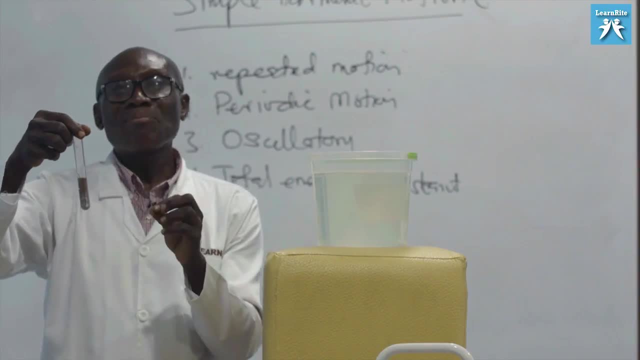 it with the right amount of any substance that we put in. it can be a substance that we put in. it can be a substance that we put in. it can be a sand. it can be less shorts, less shorts- sand. it can be less shorts, less shorts, sand. it can be less shorts, less shorts, or sand, if the right amount is put in. 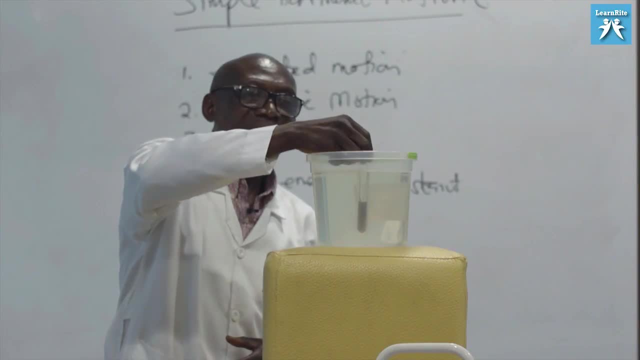 or sand if the right amount is put in, or sand if the right amount is put in it. let's see what happens. I will leave it it. let's see what happens. I will leave it it. let's see what happens. I will leave it. leave it, and the test tube suspends now. 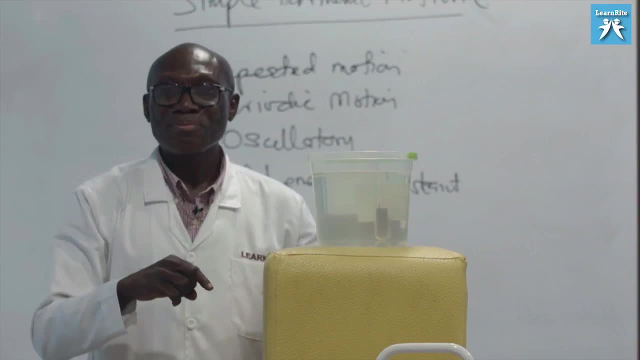 leave it and the test tube suspends. now, leave it and the test tube suspends. now we call this a suspended test tube in a. we call this a suspended test tube in a. we call this a suspended test tube in a liquid, and here we are talking about. 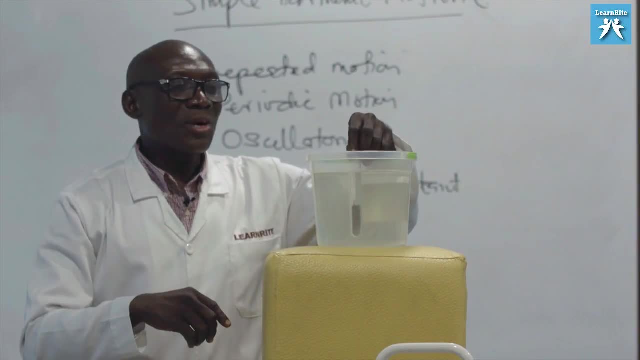 liquid, and here we are talking about liquid, and here we are talking about water. all right now, we want this test water. all right now, we want this test water. all right now, we want this test tube to show simple harmonic motion. I tube to show simple harmonic motion. I. 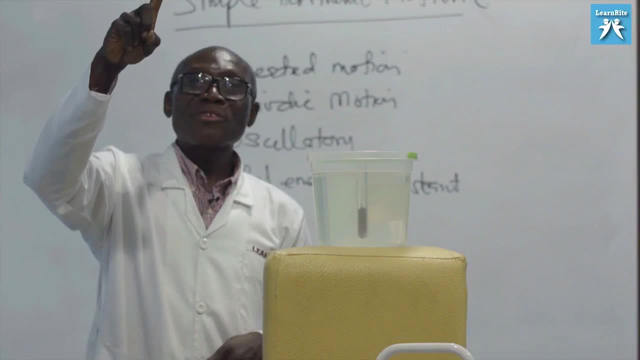 tube to show simple, harmonic motion. I hope you can see it clearly what I will hope you can see it clearly, what I will hope you can see it clearly. what I will do is to use one finger press the test do is to use one finger press the test.